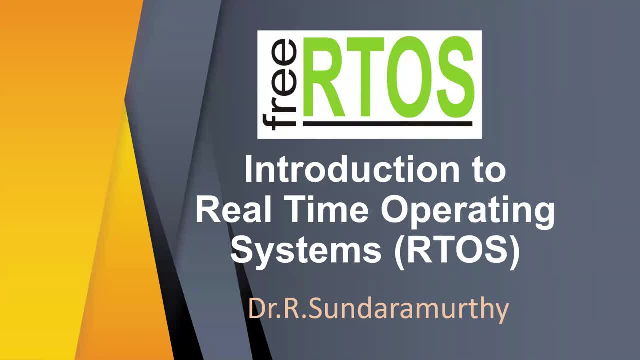 So the topic of today's discussion is introduction to real-time operating systems, or RTOS. We will see what RTOS are. what is the significance of using RTOS in an embedded system? what is the value addition that a real-time operating system brings to a 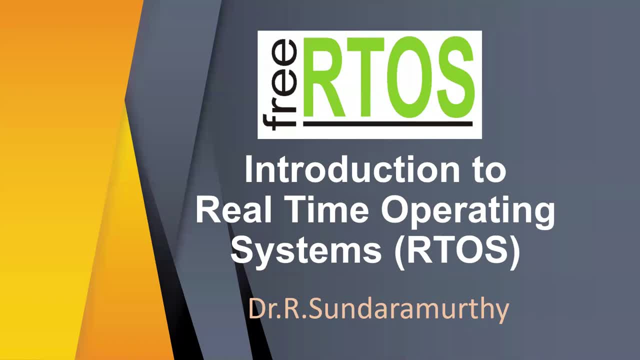 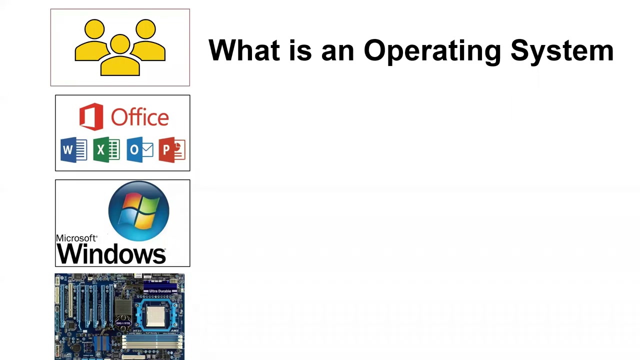 system, more specifically, an embedded system. So that is the topic of today's discussion. So this is going to be an introductory session. It is going to offer you an introduction about what a real-time operating system is. So we will proceed. Before you understand what is a real-time operating system, 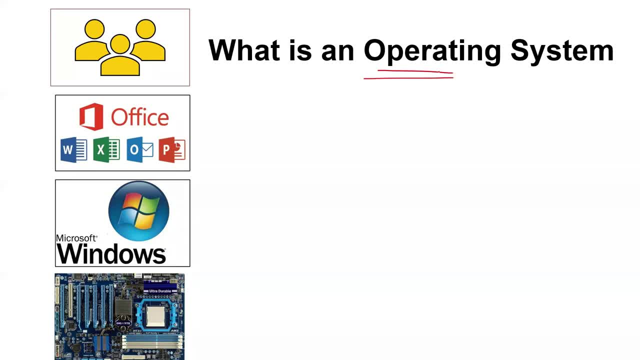 it is necessary that you should understand what an operating system is basically. So, to understand an operating system, I have given you four blocks. on the left-hand side, On the bottom-most block, you have the hardware part. Since you are dealing general-purpose operating system, let us see. this is a 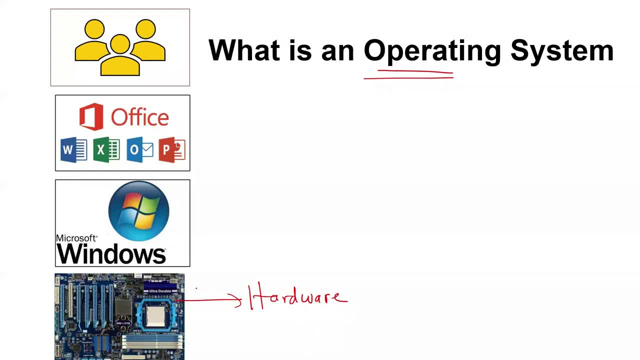 general-purpose computing system in which the underlying hardware is your motherboard with the processor. On top of that you have your operating system. On top of the operating system you have the application software, And on top of the application software you have the user. 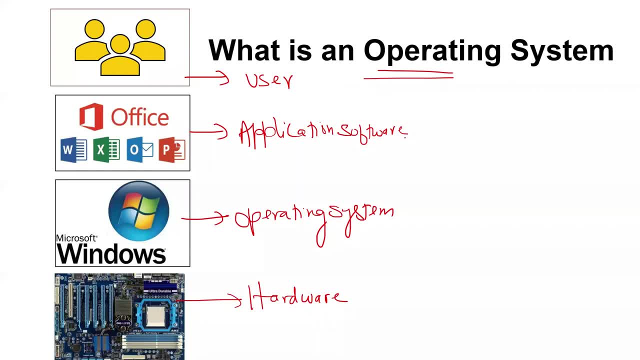 So there are four layers here. One layer is the hardware layer, the bottom-most layer. On top of the hardware layer you have your operating system or OS. On top of the operating system you have your application software And finally, you have the user. on the top-most layer. 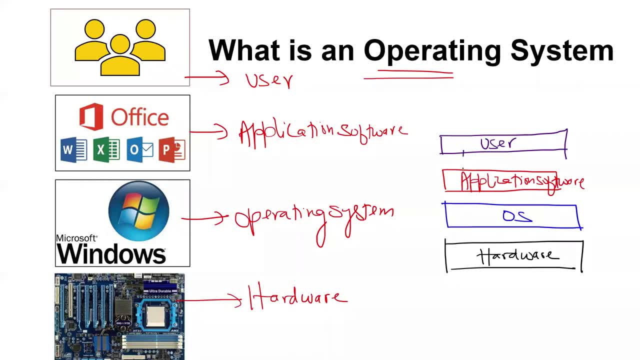 So what happens when the user is trying to interact with an application software? Say, I am using a Microsoft Word or Microsoft Excel, So what exact operation it does? basically, So, when I interact with my application software, my application software in turn pass on the information to the operating system and the operating system in turn controls the 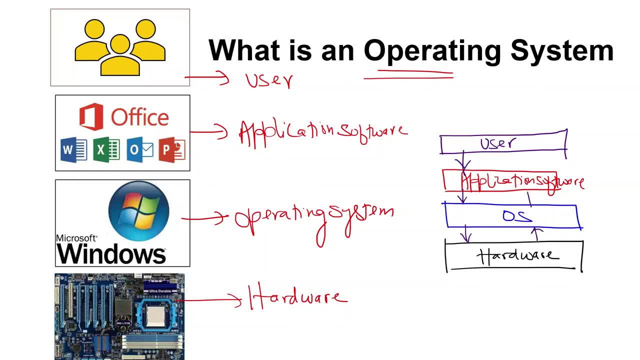 hardware. The response back from the hardware is passed back by the operating system to the application software, which is in turn communicated to the user. This is one complete cycle. So when the user is trying to interact with the application software and it is trying to get the 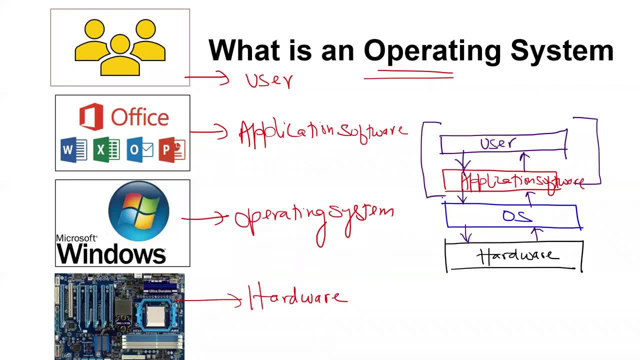 things done. basically, there is an intermediary layer between the application software and the hardware. So an operating system, in general sense it is a software. So that clarity you must have. An OS is a software which is acting as an intermediary layer between your application software and the hardware, So it is sandwiched between. 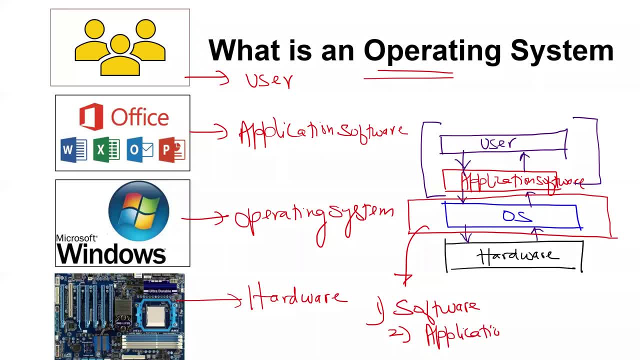 your application software and the hardware. So an operating system. in general sense it is a software which is acting as an intermediary layer between the application software and the hardware. So what is the job of this operating system? This operating system generally takes all the hardware complexities away from the application software. This operating 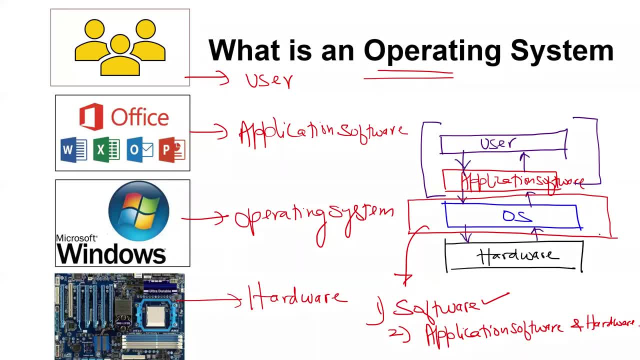 system in general sense provide set of application programming interface or APIs. These APIs are used by the application software in order to take control over the hardware, Which means the application software doesn't have to worry about the internal hardware complexities. It is taken care of by the application software. 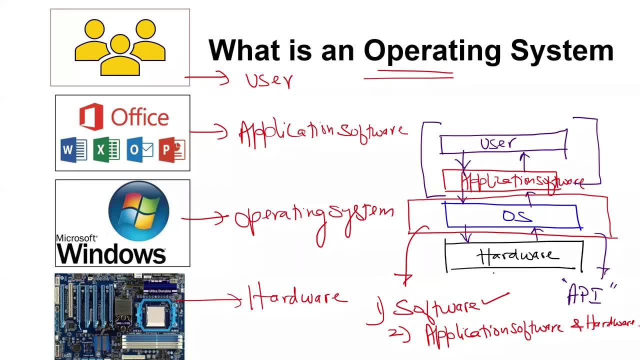 It is taken care of by the operating system. rather, The application software, on the other hand, can focus only on the application part and the entire hardware. complexity and managing the hardware, managing the resources, managing the memory, managing the IO, All the entire hardware. 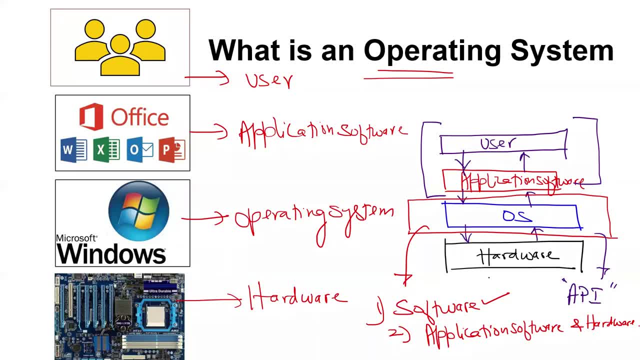 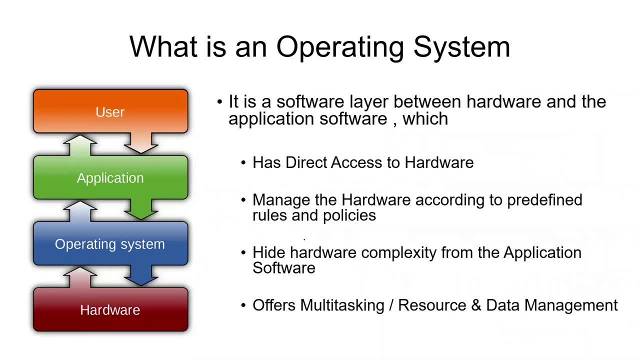 complexities are taken care of by operating system. So an operating system is an abstract layer which prohibits or which eases the application software in handling the hardware. So that is some simple thing that you can understand. So this is the simplified block diagram. I have my operating system at the underneath. So on top of that I have my operating system. 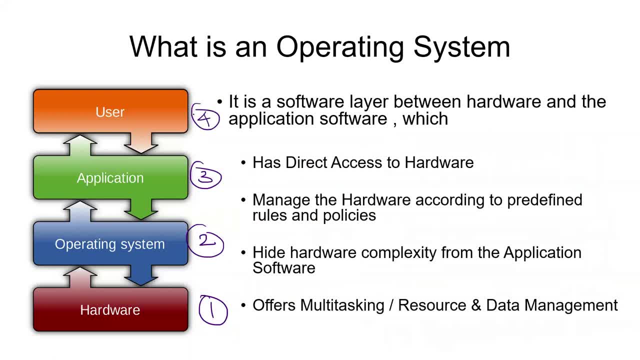 I have the application software and top of it, finally, comes the user. So in this particular architecture, what is that? something that you have to understand? So an operating system is a software layer between hardware and the application software. that I made it clear, Which number one has direct access to hardware. So if you see which software component is having, 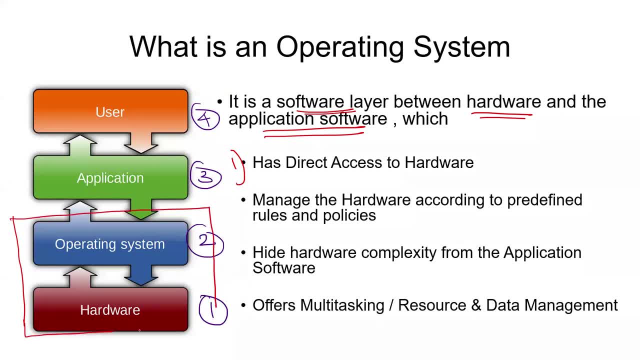 direct access to hardware. it is the operating system, not the application software. So the operating system is one which has direct access to hardware. number one. Number two: it manages the hardware according to a predefined rule and policy. An operating system, say windows operating system, manages the underlying hardware. 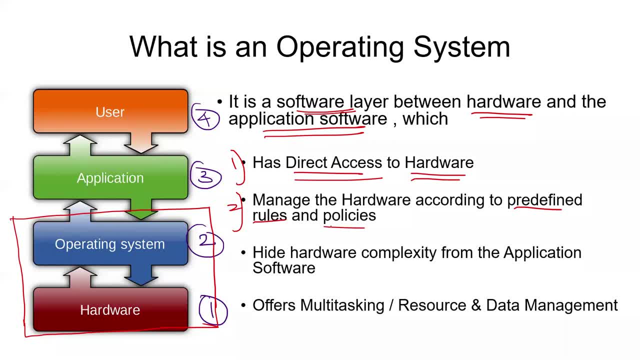 in accordance with the predetermined rules and policies of the designer of the operating system. Number three: most importantly, it hides all the hardware complexity from the application software. So this application software doesn't have to worry about the internal complexities of the underlying hardware, because it is completely taken care of by the OS. And last, 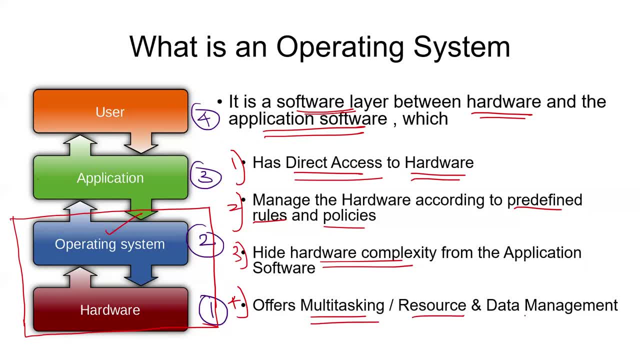 but not the least, it offers multitasking and resource and data management capability to the application software. It also offers multitasking. Multitasking is an abstract word. Multitasking means the ability to perform multiple tasks at a single instant of time. Let us see what is. 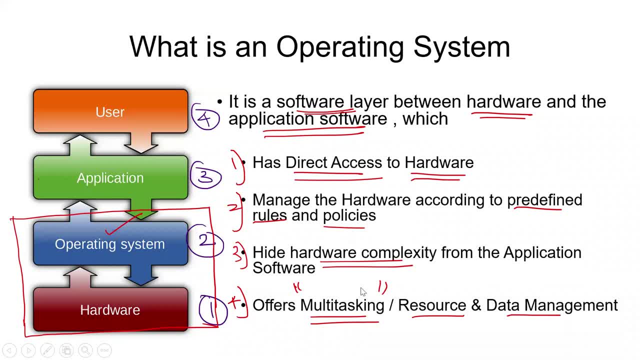 multitasking at a greater depth later, but you understand, as such an operating system can offer multitasking capability. So what we are discussing here is a general purpose OS or a gpos, which is available in all your general purpose computing systems like laptops or pcs, so on, so forth. what we are discussing here is really a. these are all examples of 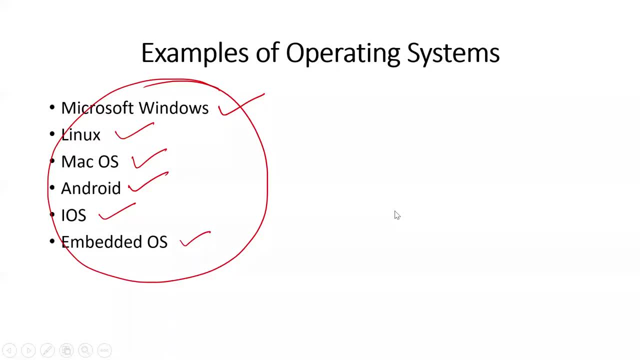 operating system: microsoft, windows, linux. these are the examples of operating systems. so microsoft, windows, linux- all these things will come under pc. android and ios will come under mobile. embedded os will come under embedded systems. so this is a generic or a general idea of an operating system. any operating system will. 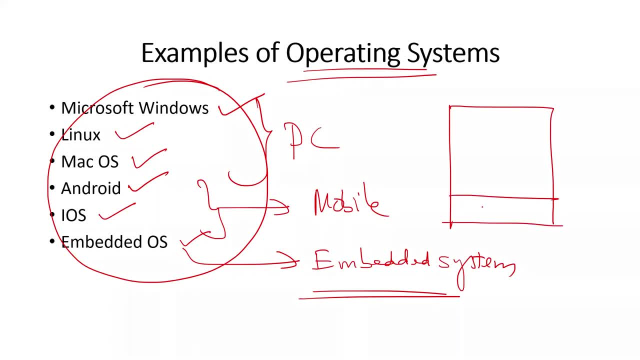 have four layers. the underlying layer is the hardware. on top of that you have an operating system. on top of that you have the application software. on top of that you have the user. so this is a generic idea, where the operating system provides an abstract layer between application. 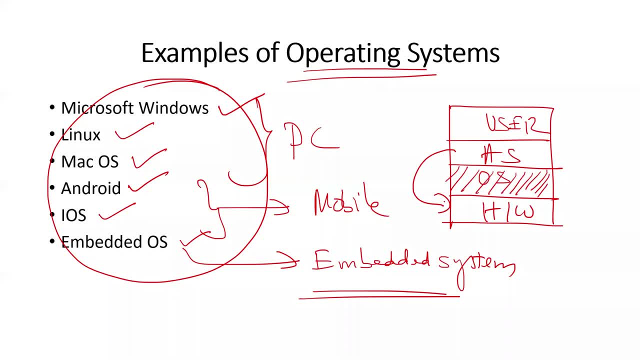 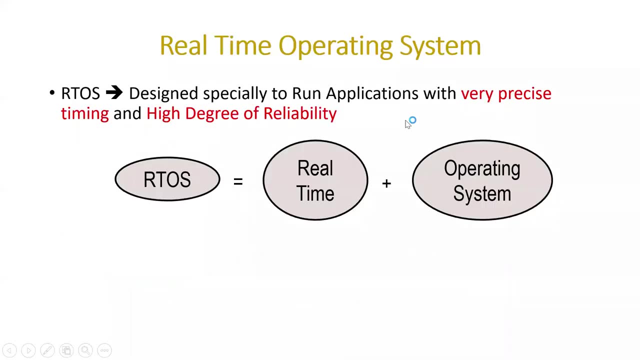 software and the hardware which hides the entire hardware complexity from the application software. so this is a general idea. now, coming back to our, coming back to our our real time operating system, what we are going to discuss in this particular class is a class of operating system called rt os or real-time operating system. 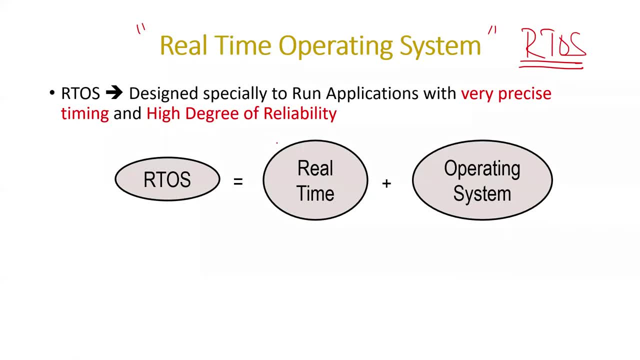 the word rt, os, or real-time operating system, consists of two components. one is a real-time component and the other one is an operating system component. the real-time operating system are arctas. It is more specifically designed to run applications with very precise timing and high degree of reliability. Reliability means it should work at any cost without failure. That is what we mean by reliability. 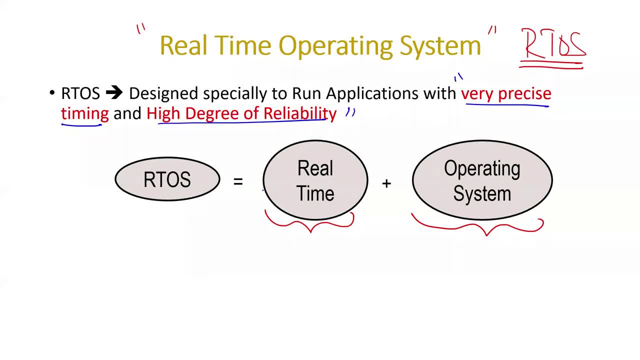 The term RTAS here refers to two components. One is a real-time component, The other one is an operating system. You know the general definition of an operating system: It is a software component that is in between your application software versus hardware. This is the general definition of an operating system. 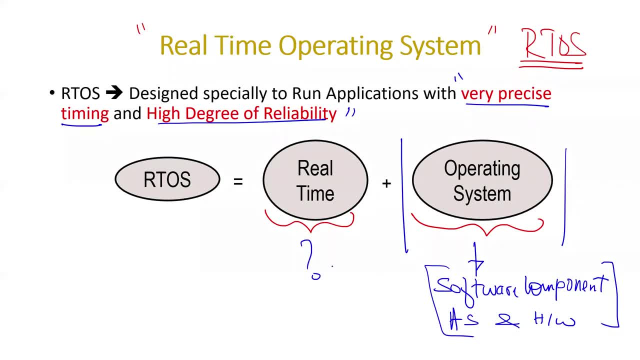 What is this real-time means? Real-time means this particular operating system should execute things with a time constraint. Time constraint means it should have a deadline. When something is executed by the operating system, the operating system should have a predetermined deadline of execution. 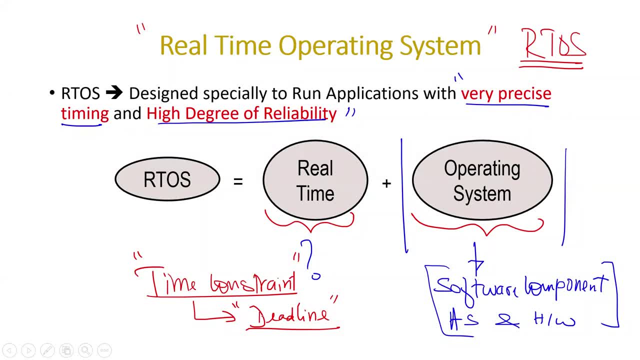 It should not be executing a task or executing an application. These predetermined time constraints are called deadlines. A real-time operating system is one which executes an application with real-time constraints. Such an operating system is called a real-time operating system. The word real-time refers to time constraint or executing something with deadlines. 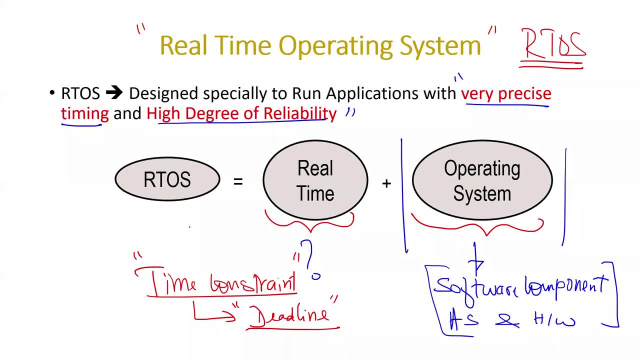 If a task is supposed to be executed in 10 milliseconds, it is supposed to be executed in 10 milliseconds, not 11 or 12.. If it executes in 11 or 12, it is not a real-time system. A real-time system is one which should execute a certain task or a certain application at a specific deadline. 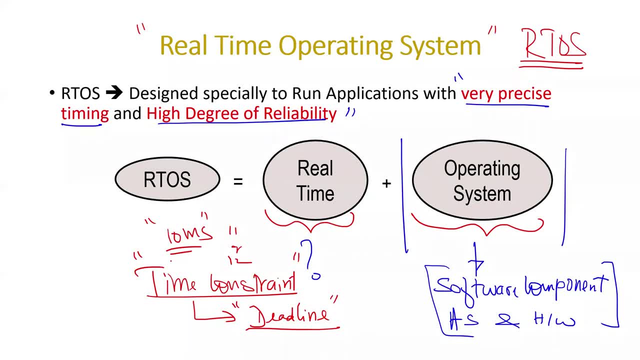 When I say deadline, it means it is supposed to finish the task before the given allocated time period. When I say a task has to be executed in 10 milliseconds, the system is said to obey real-time condition if it is about to execute that particular task well before 10 milliseconds. 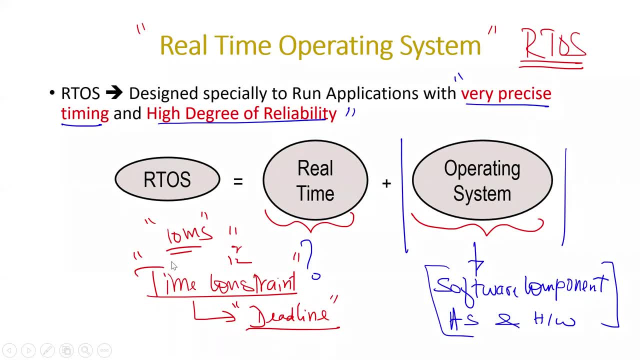 The moment it exceeds 10 milliseconds, it violates the real-time criteria. You can imagine a quiz competition: When I post a question to a team and I offer one minute for that particular team to answer that question, the team is supposed to answer that particular question well before one minute. 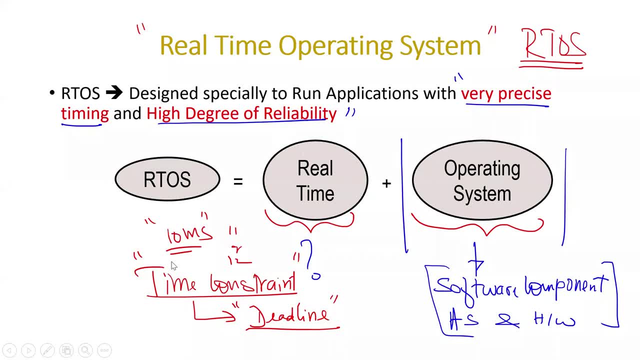 Only then that particular answer is considered as a correct answer. Which means in a quiz, if that particular team is able to tell me a correct answer, but unfortunately not in one minute, but they take two minutes- then that right answer is considered to be a wrong answer. 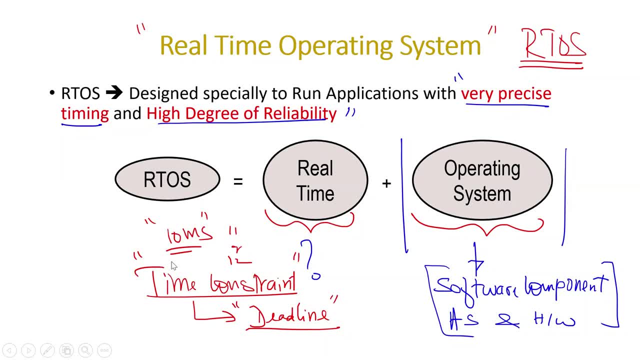 That is a similar situation here. In a real-time situation or a real-time system, a late answer is always a wrong answer. A late answer is a wrong answer means even if it is executing certain things, even if the computational results are correct. 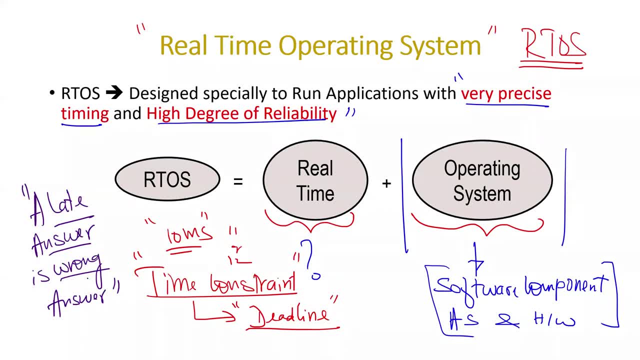 unless otherwise it delivers the result in a specific deadline, it is not considered useful. The answer is considered to be a wrong answer. That's what it means. So the word real-time means an operating system's capability to deliver the result with a specific time constraint. 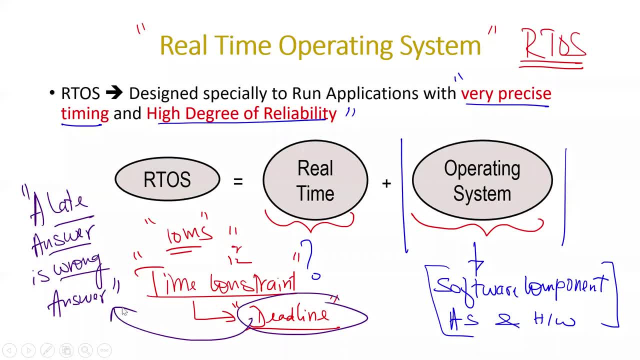 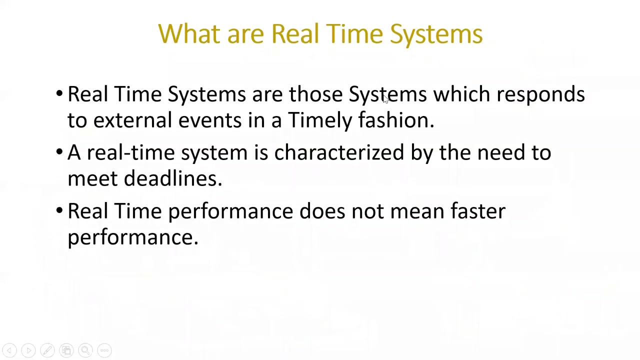 General operating system is not meant to be functional that way. Their priorities are different. A real-time operating system is revolved around this. real-time criteria. All of you are with me. Are you following what is going on in the class? Okay, 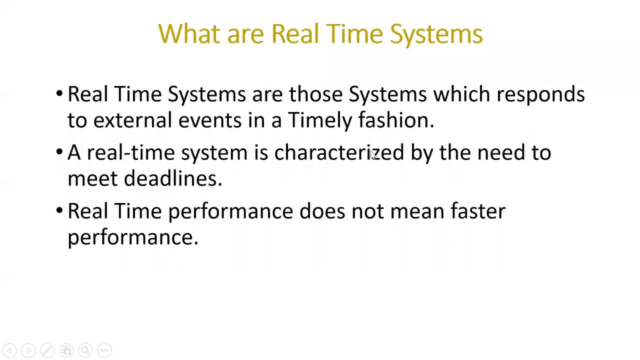 So what are real-time systems means? What is the definition of a real-time system? What real-time system means? Real-time systems are those systems which responds to external events in a timely fashion. They spontaneously respond for external events in a timely fashion. 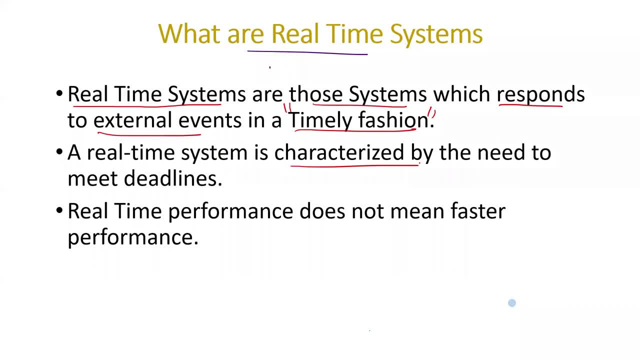 Real-time system is characterized by the need to meet deadlines. They are expected to work within a specific time frame. They are expected to deliver results within a specific deadline, And a common misconception is that real-time performance does not mean faster operation. Any system which is operating at a faster rate is not considered as real-time. 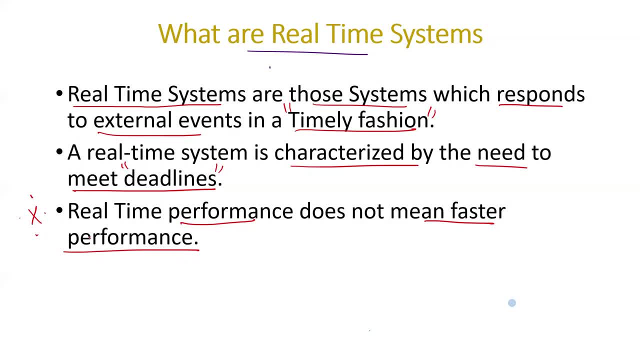 A real-time means it should have the ability to complete things within a specific deadline. not necessarily it has to work at faster rate. So if a system works at a faster rate still it is not completing the deadline, is not considered a real-time system. 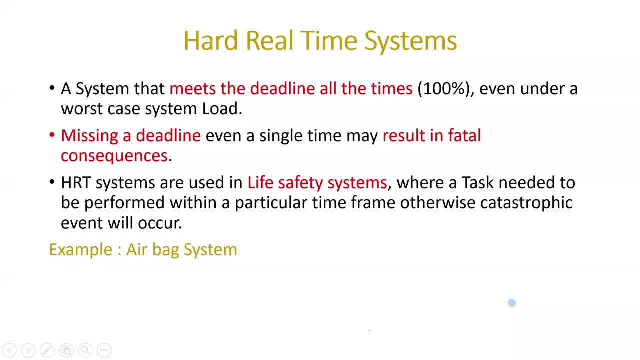 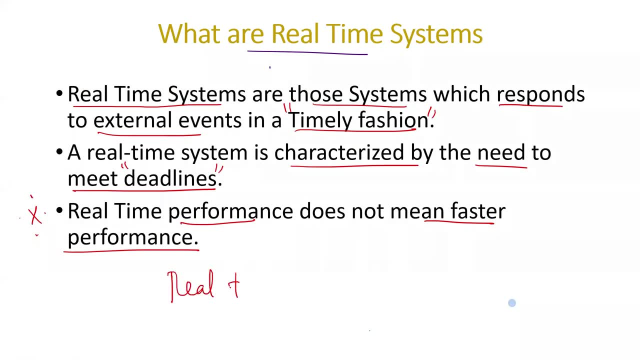 So that clarity you should have. There are two types of real-time systems that we deal here. One real-time system is called hard real-time system. The other one is called soft real-time system. You all know what real-time system is. Real-time system means that particular system should have a deadline. 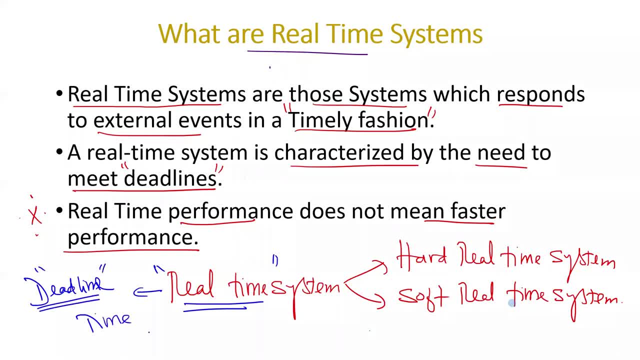 The system should work on a specific time frame. Such a system is called real-time system. What if the system misses the deadline? That categorizes hard real-time and soft real-time system. Both systems are real-time systems only. What if they miss that deadline? 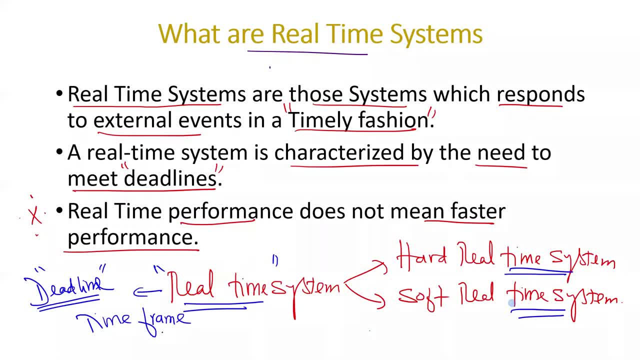 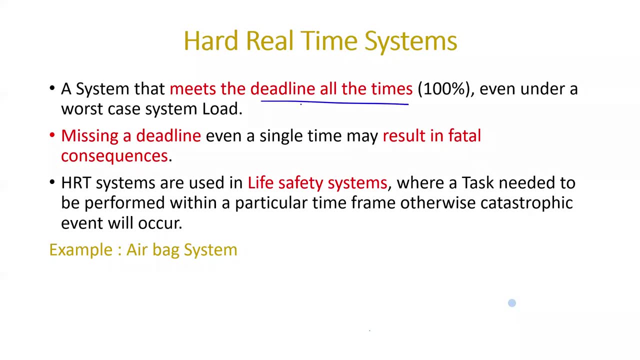 What if they are not able to cater the time frame? What if they miss the deadline in certain cases, occasionally or frequently? What happens then? Hard real-time system means the system should meet the deadline all the time. 100% of the time the system should meet the deadline. 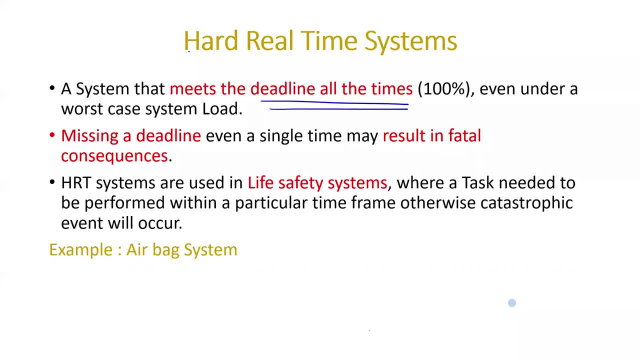 There is no room for missing a deadline in hard real-time systems. So hard real-time systems are characterized by meeting the deadline all the times, 100% of the time. it has to meet the deadline. Even in the worst case situation it has to do that. 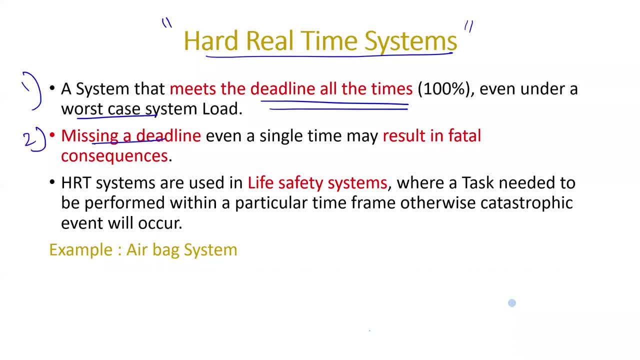 That is the number one. Number two: Missing a deadline results in fatal consequences. It may lead to loss of life, A catastrophic outcome, Very dangerous outcome. Such systems are called hard real-time systems. Hard real-time systems are those where missing a deadline may lead to a fatal consequence or loss of life. 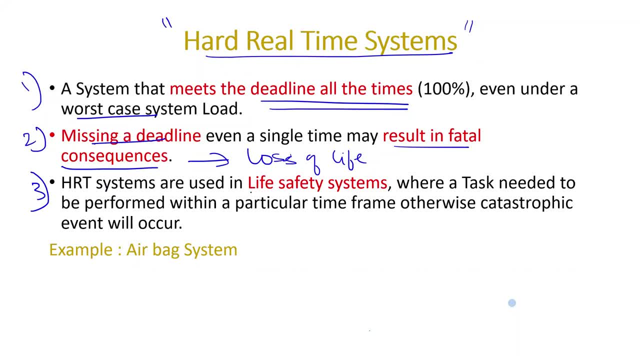 Number three: Hard real-time systems are used in life safety systems where tasks needed to be performed within a specific time frame. One beautiful example I always tell students is an airbag system. When you are traveling in a car and the car makes an impact somewhere and it releases an airbag. 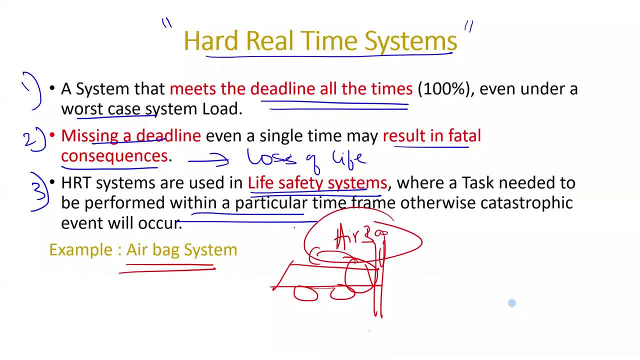 When the airbag is released, it is expected to release that airbag in a specific time frame, In a specific millisecond time period. If it is not releasing in that specific millisecond time period, then a late answer is a wrong answer in this case. 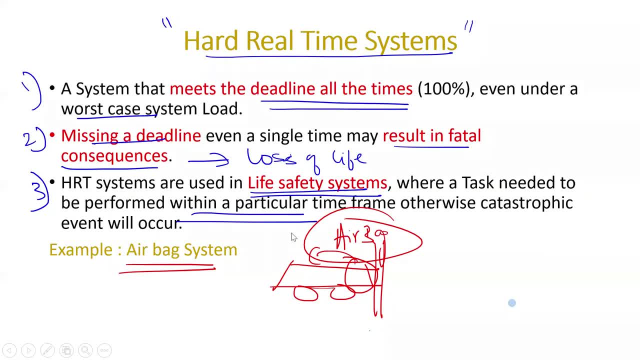 There is no point in releasing the airbag. It is not acceptable if the airbag is releasing after one minute or so. So you cannot live with that kind of a system because by the time it releases, the patient is already gone, The driver is already gone. 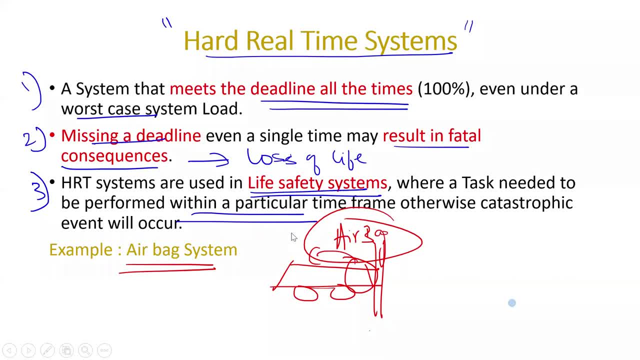 So such systems result in loss of life if they miss a deadline. Such systems are called hard real-time systems, So missing a deadline results in loss of life- Loss of life or an unwanted outcome. So that is what you mean by hard real-time systems. 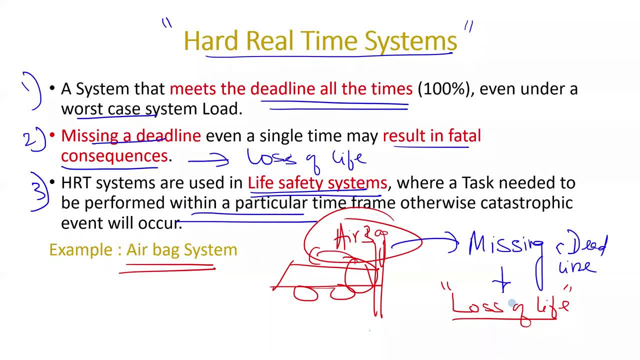 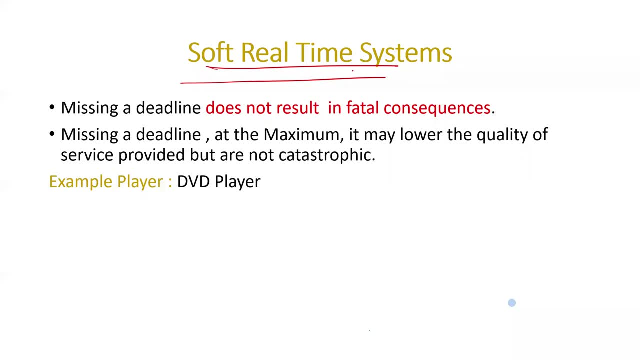 Hard real-time systems are not expected or they should not miss a deadline at any point in time. 100% of the time they are expected to meet the deadline. Such systems are called hard real-time systems. What are soft real-time systems? Soft real-time systems are those kind of systems where missing a deadline does not result in a fatal consequence. 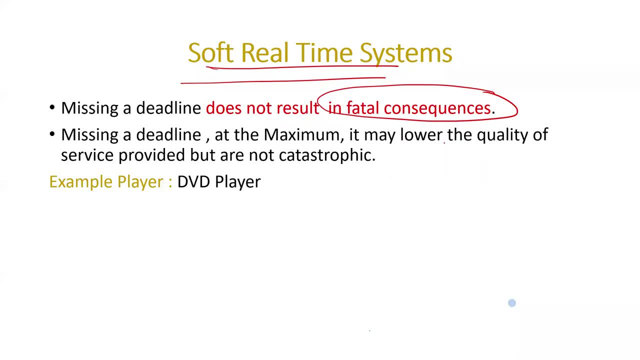 Whereas missing a deadline may deteriorate or lower the quality of service, The system's service may deteriorate or degrade, but it will not result in a fatal consequence. It may not result in loss of life kind of a situation. Say, for example, DVD player. 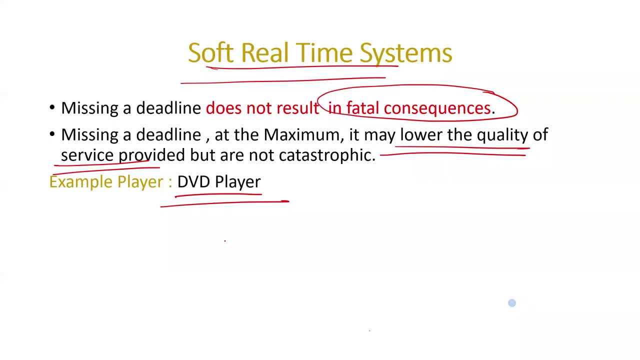 I have a DVD player. This DVD player is used for playing videos. Playing videos means it is expected to stream a specific number of frames per second. Let us say it is streaming at 12 or 24 frames per second. In the due course of streaming the frames per second, let us say it is missing a frame. 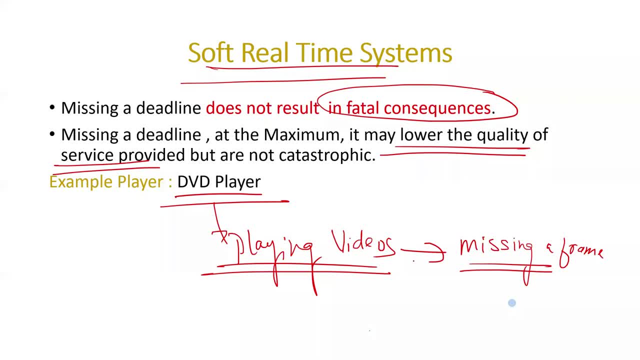 Or it is missing a deadline in playing that particular video. This is not going to lead to any unwanted outcome. Probably it may result in an unpleasant or it may give a small jitter in viewing the video. It may be unpleasant for a fraction of second. 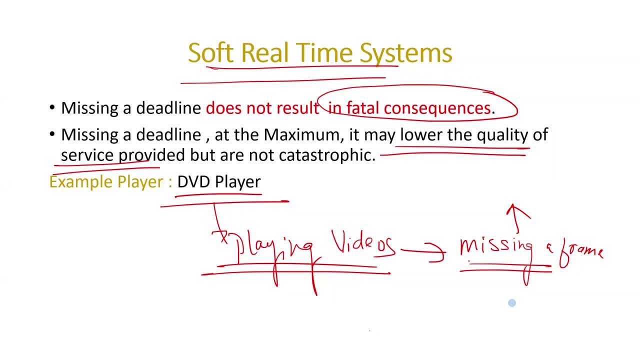 But then it is not going to be a very fatal consequence that somebody is going to die because of that. So that is something that you have to understand. A soft real-time system is one where missing a deadline is acceptable. Okay, that's fine. 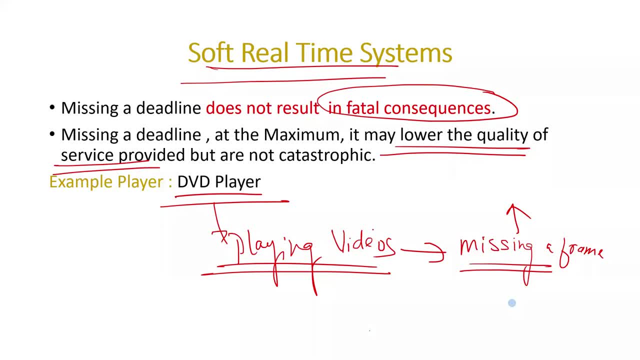 It is not that the system should be designed that way. I am not telling it. But missing a deadline is not resulting in a fatal consequence. Rather, it degrades or lowers the quality of the service that that particular product is offering to you. Such systems are called soft real-time systems. 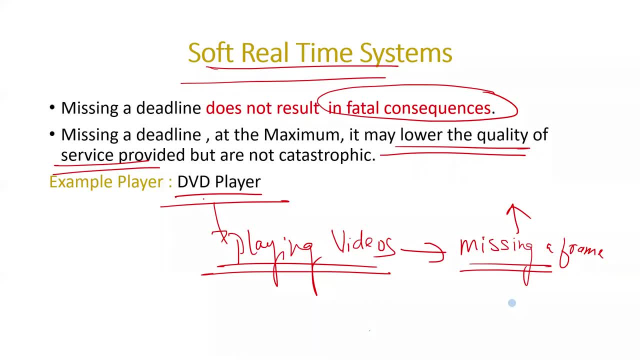 Most multimedia devices: digital cameras, VCD players, musical systems, website services. IRCTC is a real-time system. IRCTC is able to execute things on real-time. It is able to deliver results on real-time basis, But it is a soft real-time system. 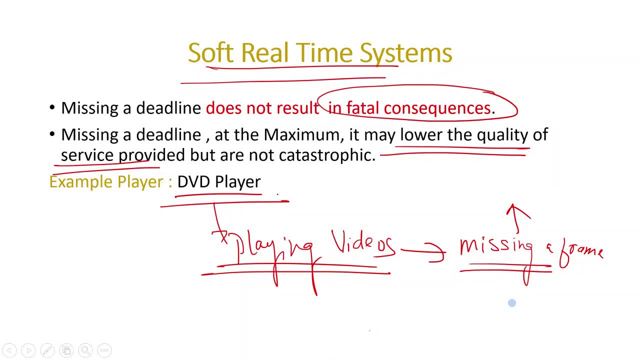 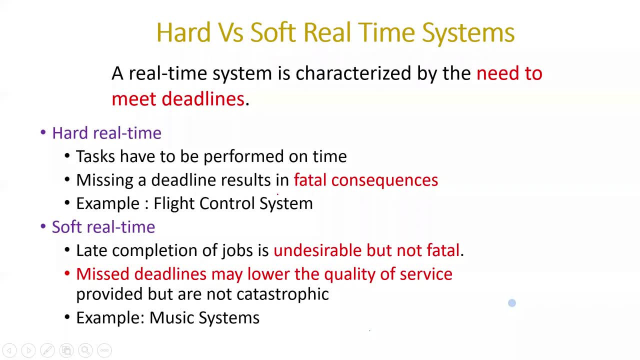 Okay, Because the outcome of that may not be meeting the deadlines all the time, Okay. So that is something that you have to understand. So you have to clearly understand the difference between hard versus soft real-time system. Hard versus soft real-time system means in hard real-time systems, the tasks have to be performed on time. 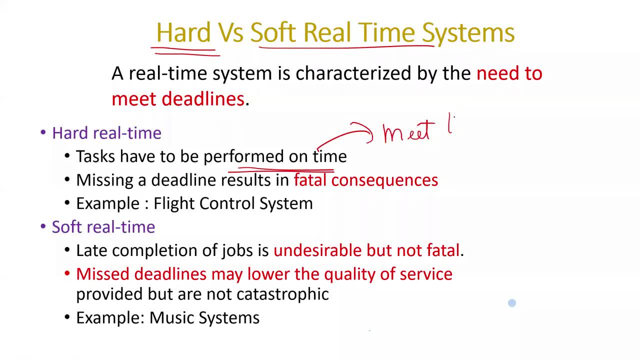 They have to meet the deadline 100% of the time. Missing a deadline result in fatal consequence: Loss of life. They can give lot of such examples: Flight control systems, What is soft real-time system, Late completion of job result in undesirable output, but not fatal. 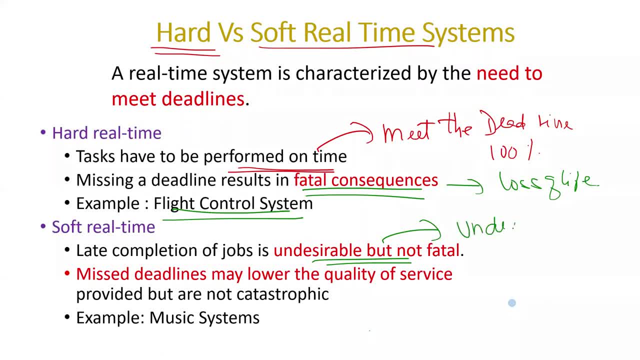 You know, undesirable. Undesirable means the quality of the service is going down, but it is not fatal. Missing the deadline may lower the quality of service, but it is not catastrophic. Example: all multimedia systems will come under soft real-time systems. 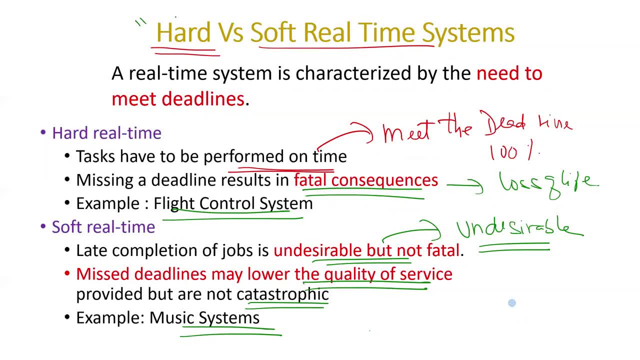 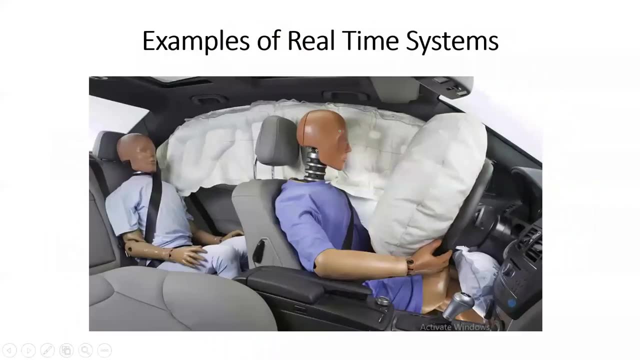 So you have to very clearly distinguish what is hard and what is soft. Hard real-time systems are those systems where meeting the deadline in 100% of the times is mandatory. There is no relaxation. Soft real-time systems: it is okay if it could miss few of them. 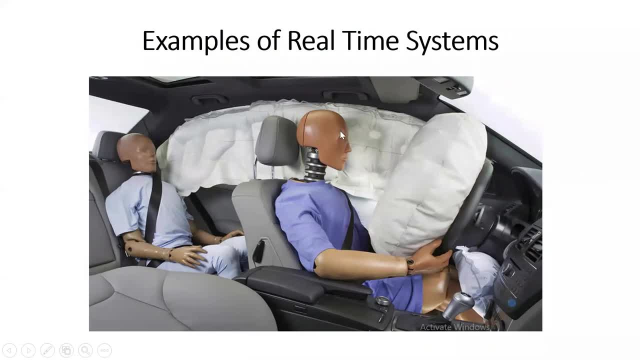 So let us see few examples of real-time systems and which classification it fall under. First one is an airbag system. When a driver is meeting an accident, the system is releasing an airbag, typically within a millisecond of the impact. So such a system is classified under hard real-time system. 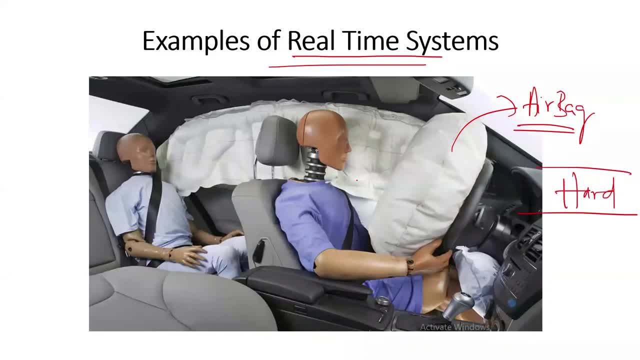 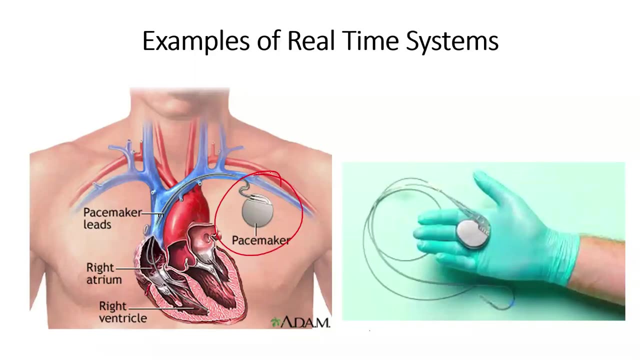 Why it is called hard real-time system, Because it may result in loss of life of the passengers as well as the driver. So this is a clean example one can give for a hard real-time system. The other example that I can give for a hard real-time system is a pacemaker. 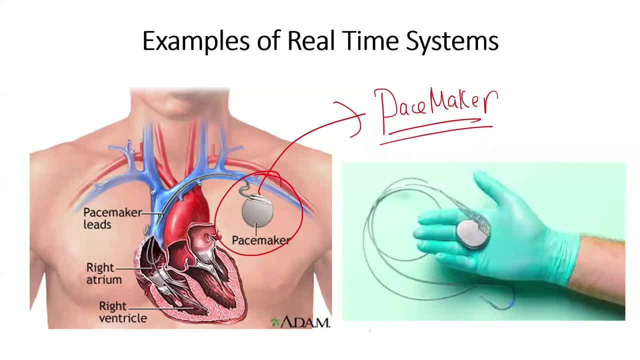 Pacemaker is an electronic equipment that is normally injected slightly below your collar bone That supply the electrical pulses for your heart, more specifically the ventricles to regulate your heart pulses. Sometimes it may be lower, sometimes it may be higher. So in order to regulate your heart pulsing, we need to have a pacemaker. 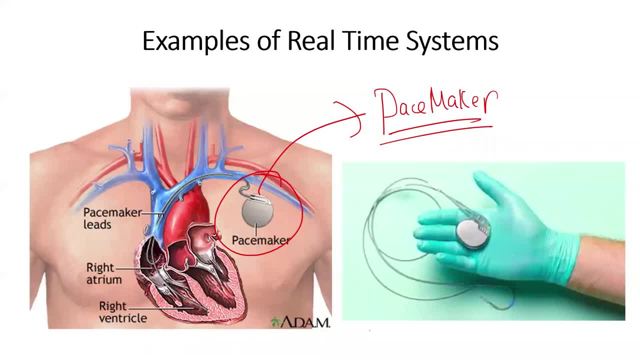 This pacemaker device supplies electrical pulses to your ventricles In order to regulate the heart pulsing. So this is yet another example one can give for a hard real-time system, Because it is expected to work at a specific time frame and it is expected to deliver the pulses to the heart at a predetermined interval. 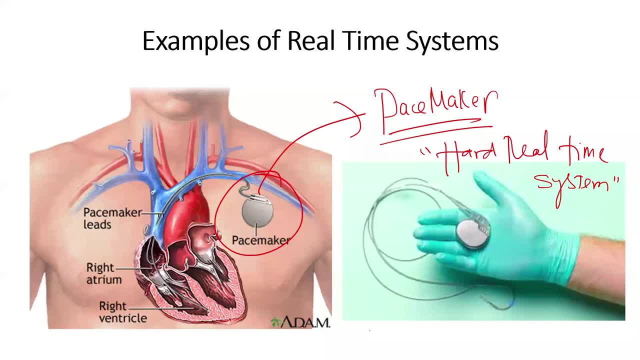 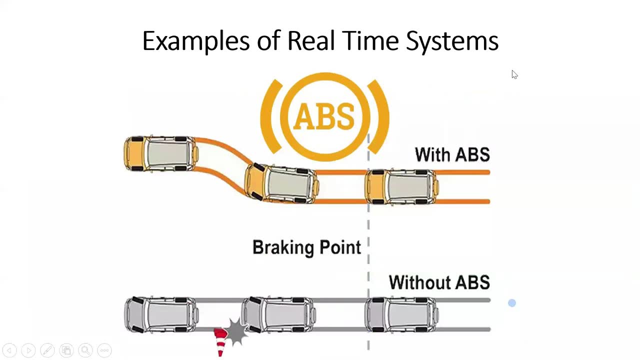 Failing which it may be fatal for the patient. So that is yet another hard real-time system. The other hard real-time system can be ABS or anti-lock braking systems. This anti-lock braking systems or ABS systems are most predominantly used in four wheelers. 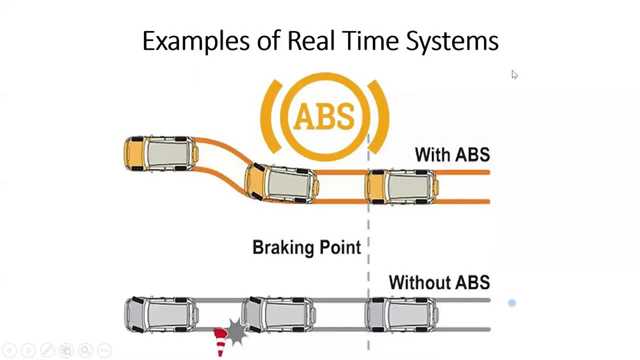 See when you are driving in a skiddy surface or when you are travelling at a very fast pace And when you are suddenly applying a brake which is beyond the gripping capability of your tyre. When you have an ABS or anti-braking system, you still have the control to steer over the vehicle and establish a normal control over the vehicle. 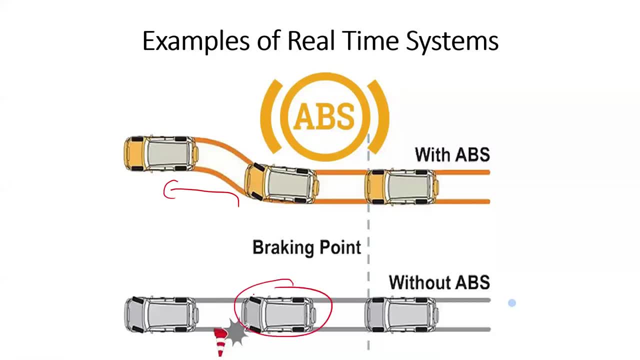 Without ABS, the vehicle will collapse and it will skid in the road And it will fall, It will skid in the road and most likely it will end up in an accident. So ABS is again yet another real-time system which measures the speed of all the four wheels. 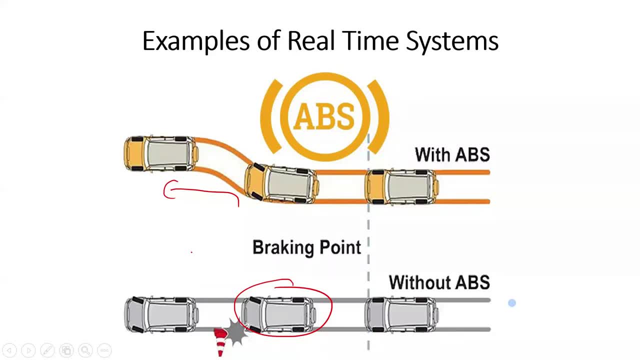 And in the event of a speed drop in any particular wheel, the ABS system will automatically take control over the brake cylinders and then control them accordingly. So ABS or anti-braking systems, anti-brake locking systems are yet again another real-time systems. 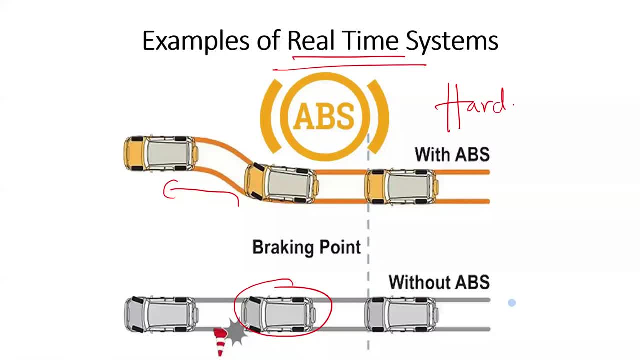 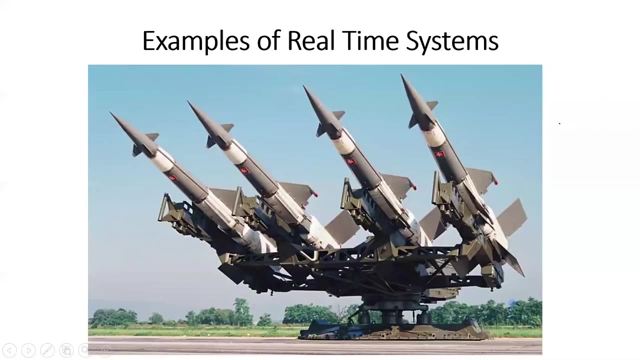 Which again come under hard real-time systems. Anti-lock braking systems are present in most modern day cars. Missile control systems- again hard real-time systems. The way they lock a target, the way they track them and they precisely hit them is entirely time controlled. 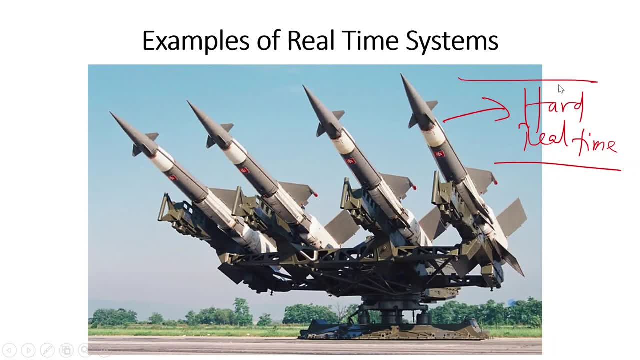 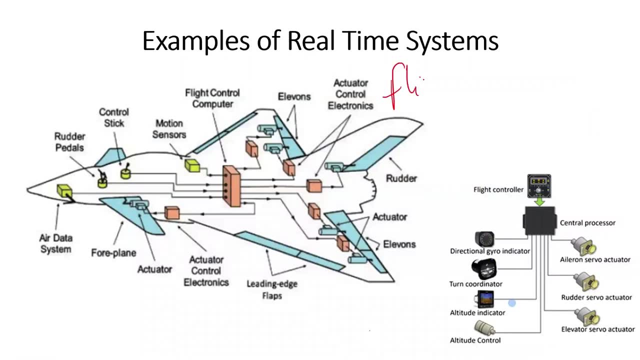 It is a hard core embedded system Again comes under hard real-time category. Flight control systems: Again comes under hard real-time category. It dynamically acquires sensors information, calculates what is the altitude it has to control and take decision action in order to control all the actuators inside the flight. 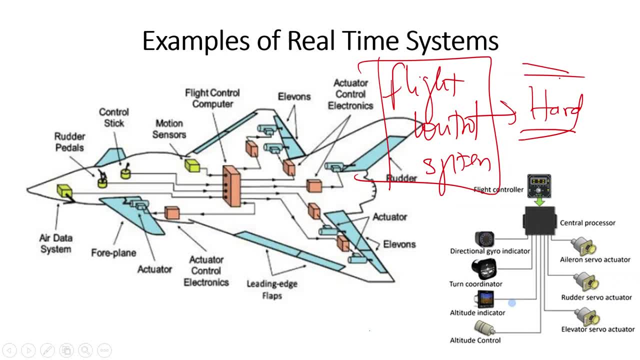 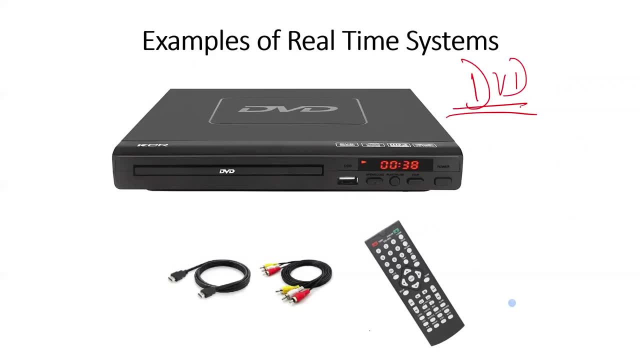 So it is yet again another hard real-time system: A DVD player. This is a real-time system which is supposed to stream your videos at a particular frame per second, But still, if you are going to miss a particular deadline, you are not going to have any loss of life or any catastrophic outcome. 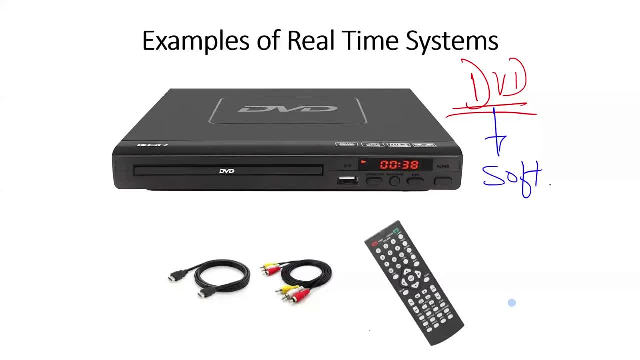 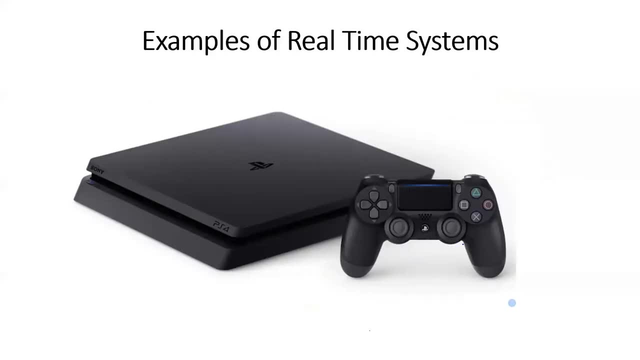 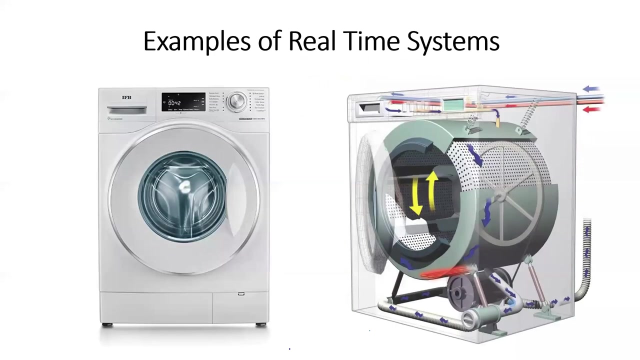 So hence it comes under soft real-time category. Game consoles, Again, comes under soft real-time category. But still, if you are going to miss a particular deadline, you are not going to have any loss of life or any catastrophic outcome. The finally comes under soft real-time category. 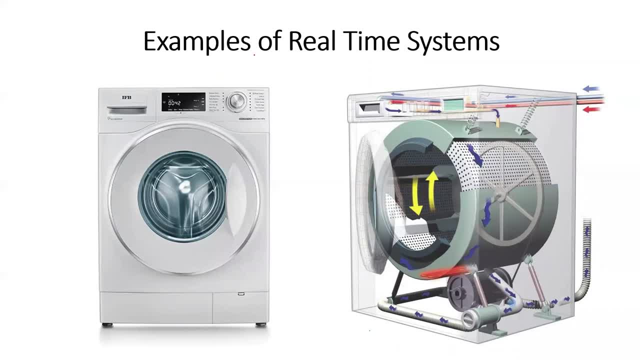 The washing machine Again comes under soft real-time category, But still, if you are going to miss any subsequenthel kilograms, an issue arises in the mind of the machine. Same for a hard real time regime. No doubt that it is a real time system, but missing a deadline here doesn't result in. 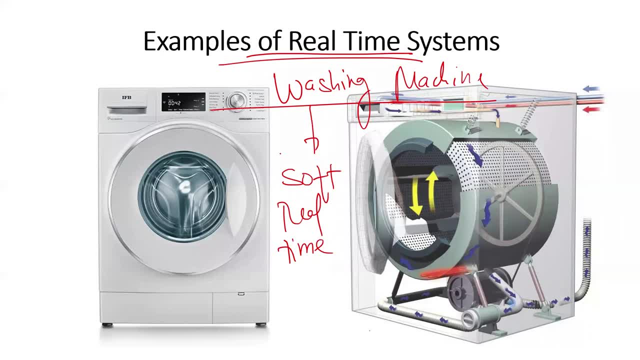 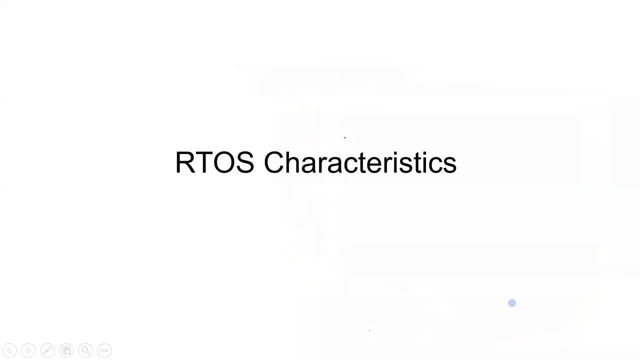 any catastrophic or loss of life. So that is still a soft real time system. So these are all some of the examples that I wanted to give you: hard versus soft real time systems In general. for hard real time systems, meeting the deadline has to be done in 100% of the. 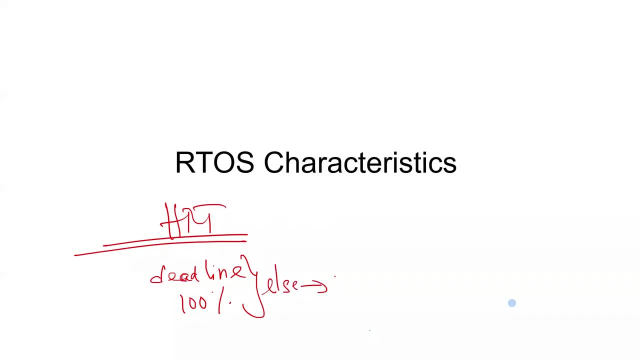 cases. else it will result in loss of life For soft real time systems. missing a deadline means quality of service, It is going down, but it doesn't result in unwanted outcome. So this is something that you have to understand. All of you are with me. 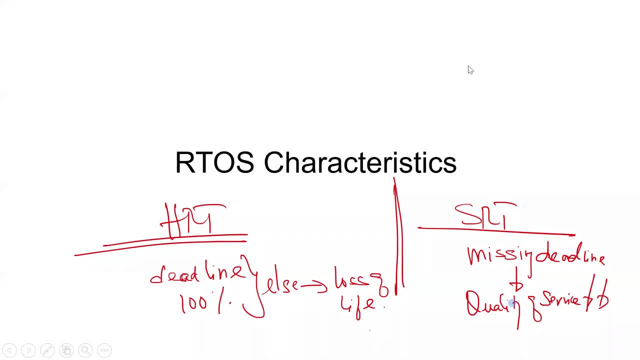 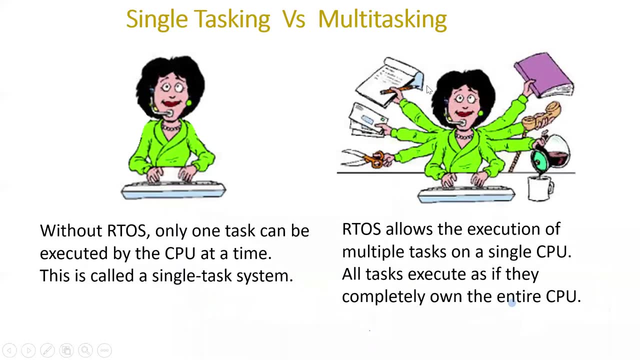 So far clear. What are the important characteristic features of soft real time systems? What are the important characteristic features of soft real time systems? What are the important characteristic features of soft real time systems? So procedure 1 of a real time operating system. 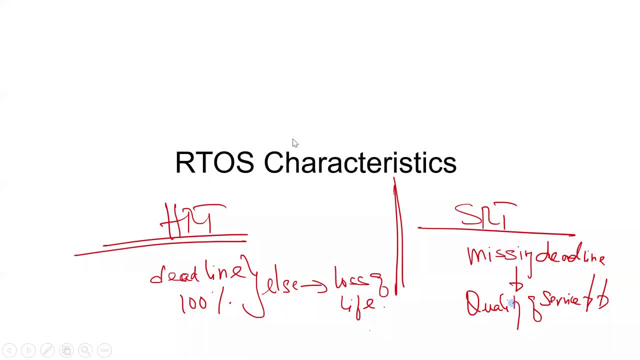 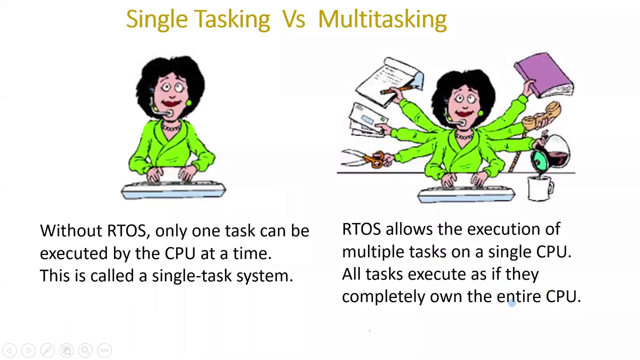 Out-of-s acknowledgement of passive� virus or hemosa partner. Hard task characteristics- garder꼬- Its what we are going to discuss now. A real time operating system has a certain unique characteristic feature. One of the important characteristic feature of a real time operating system is the ability. 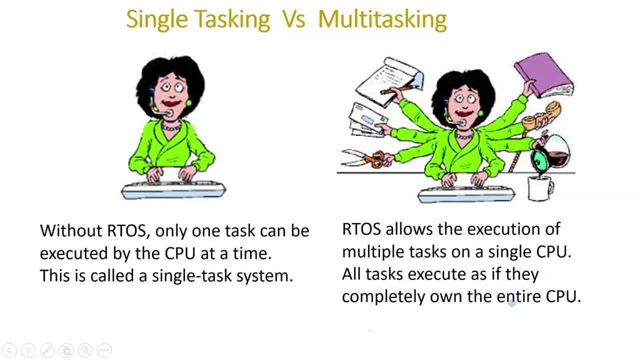 to perform multiple tasks at the same time. Multi-tasking, capability, multitasking and what is multitasking? Both of them are single individuals, which means they have only one CPU. CPU here refers to brain. Here also there is only one CPU. So 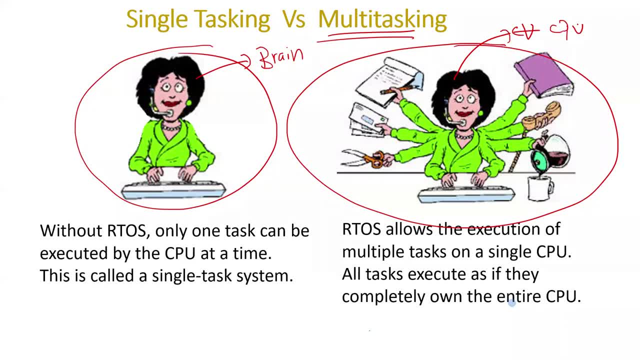 practically in a single CPU, you can do only one task, So that is the natural way of doing it. If I have only one CPU, I am currently taking class for you, so that is the only task I can do. On the other hand, if I am able to do multiple tasks when I am doing or focusing- 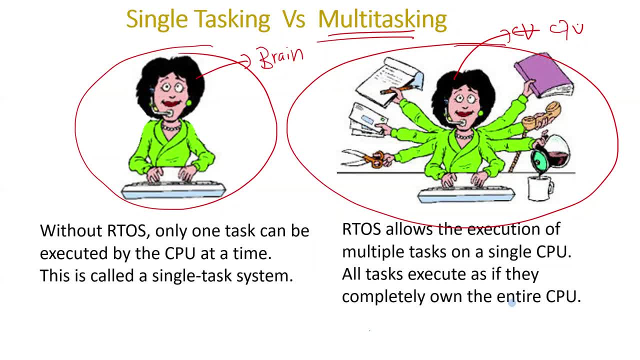 on one particular application. I said to perform multitasking, But it is against the natural flow in which a CPU works. A single CPU can allocate time for only one task. But if the single CPU is able to perform multitasking, then it is against the natural flow in which. 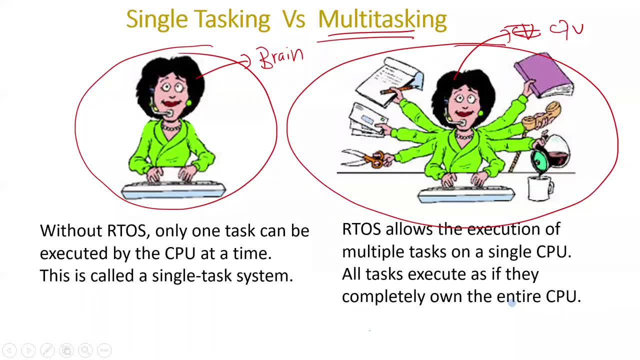 a CPU works. A single CPU can allocate time for only one task. But if the single CPU can allocate time for only one task, But if the single CPU can allocate time for only one task, But if a CPU is said to perform multiple tasking, there should be some level of trick or some level. 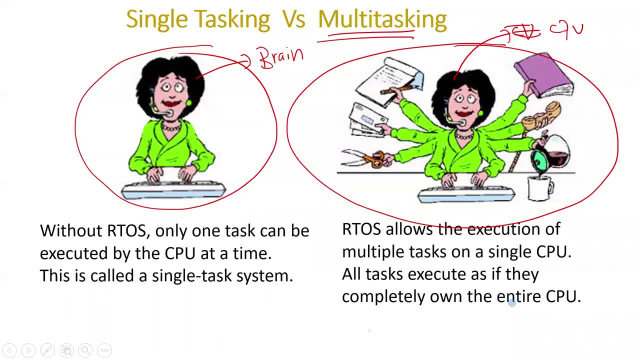 of computational manipulation going on underneath in order to make someone to believe that the processor is performing multiple tasks. So that is some kind of a software trick. I would say So there is a dedicated software engine that is sitting inside your processor that does this trick for you. 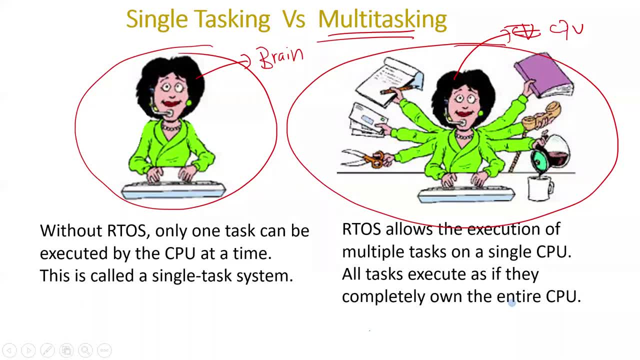 That software which does this trick of making somebody to believe that a single processor is performing multiple tasks is called a real-time operating system. The job of the real-time operating system is to share a processor for multiple tasks, and it gives the ability to the processor to execute multiple tasks by time-sharing its resources and time in an effective manner. So that is what it does effectively. 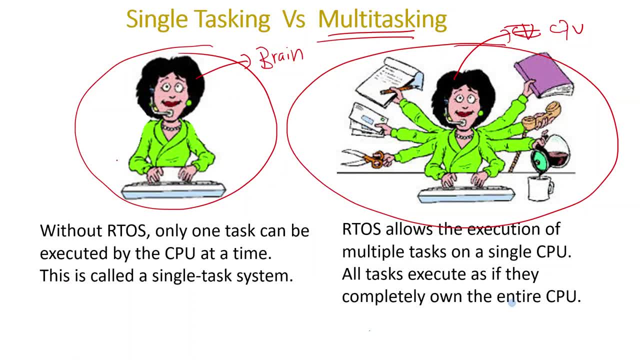 So this is our conventional embedded system. So far, what we have been doing is a single-tasking system. Single-tasking system is a single-tasking system. Single-tasking system means what We don't use, any R-tasks, Only one task we are going to execute in a cyclic manner. That is called a single-task system. 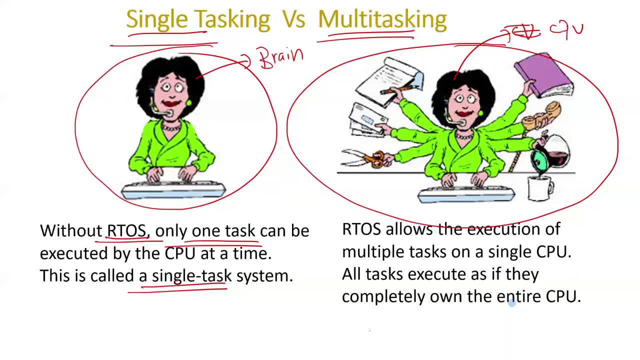 A microcontroller is able to execute a single task over and over in a cyclic manner. That is what we have been doing so far. So what we have been discussing so far is a single-tasking system. Don't confuse between functions that a microcontroller performs versus tasks. 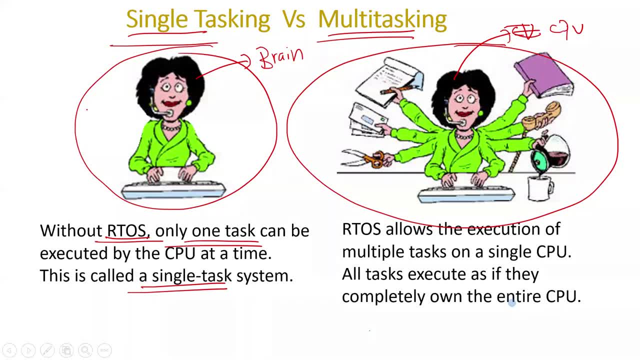 Okay, There is a clear difference. for that I will explain you that. Multi-tasking means the microcontroller is able to execute multiple tasks with a single CPU. That is the key thing that you understood. A multi-core CPU naturally has the capability to execute multiple tasks. That is different. 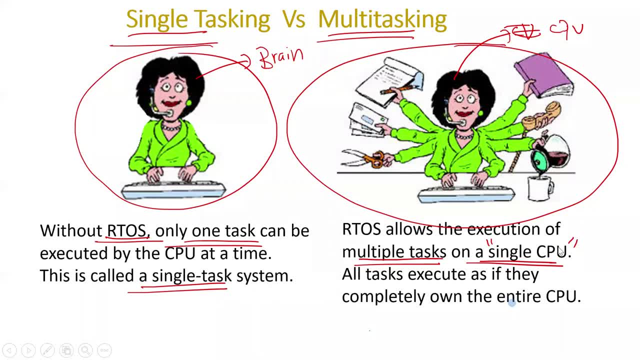 With a single core or a single CPU. if the microcontroller is able to execute multiple tasks, then it is said to have a multi-tasking capability. That multi-tasking capability is offered by R-tasks, not by a native programming. Okay, 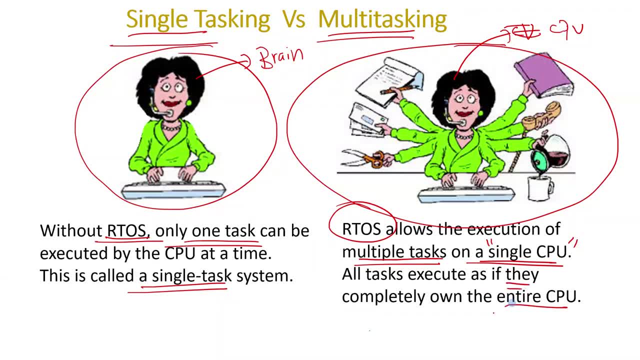 So all the tasks execute as if they completely own the CPU. This is an ability that an R-task offers to each and every task. Each task takes ownership of the CPU for a predetermined time, And once that is done, that ownership is given to somebody else. 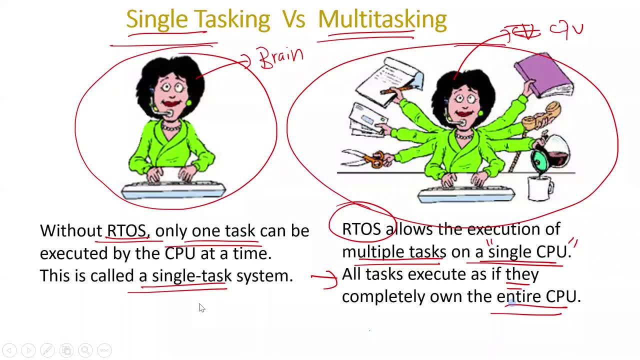 So all the tasks take the ownership of a task And once that is done, that ownership is given to somebody else. So all the tasks execute as if they completely own the CPU. That is the key thing that you understood. So there is a key component that is present inside R-task called a kernel or a scheduler. 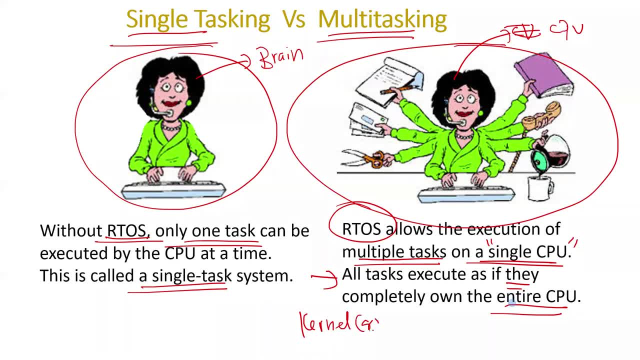 So there is a key component that is present inside R-task called a kernel or a scheduler, which does the job of sharing the processor's time to which task at what time instant. which does the job of sharing the processor's time to which task, at what time instant. 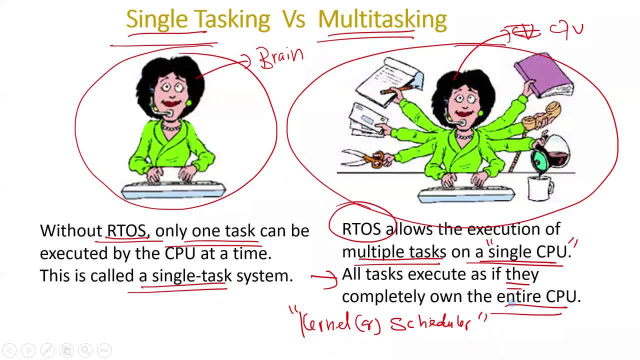 So that is taken care of by the kernel or the scheduler of the R-task. but in general, in a single tasking system the CPU can perform only one task. in multitasking system, multiple tasks can share the time of the processor in a predetermined manner so that the processor is able to cater multiple. 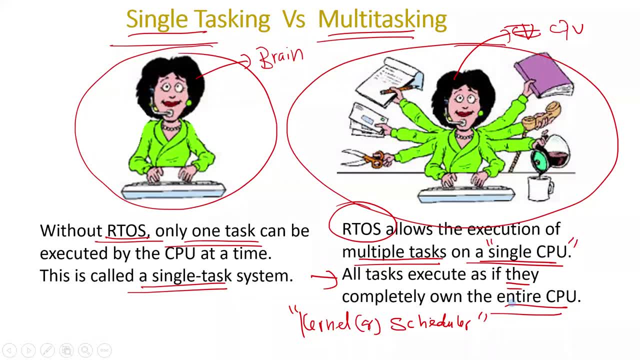 tasks at the same with the same CPU. so that is the difference between that. so what is the difference I am trying to tell here? this is with OS. this is without OS. this is without OS. I mean RTOS. this is with OS. with RTOS, with the single CPU, you have the power to execute multiple tasks. 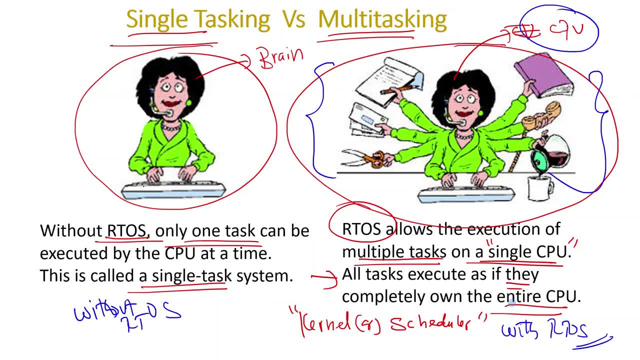 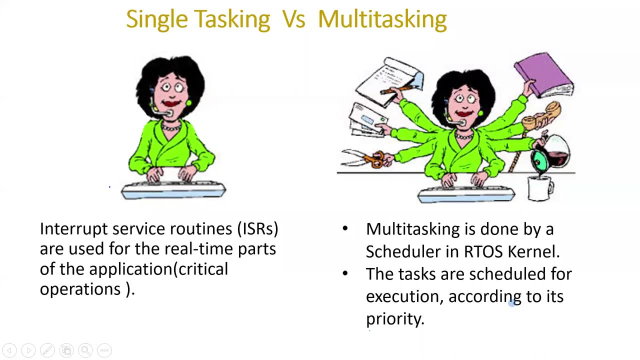 without RTOS? you don't have that capability. you can only perform only one task. that is what it means. so what is the power of our task? that brings to your table is what I am trying to explain here. there is a way of performing multitasking even in the absence of our 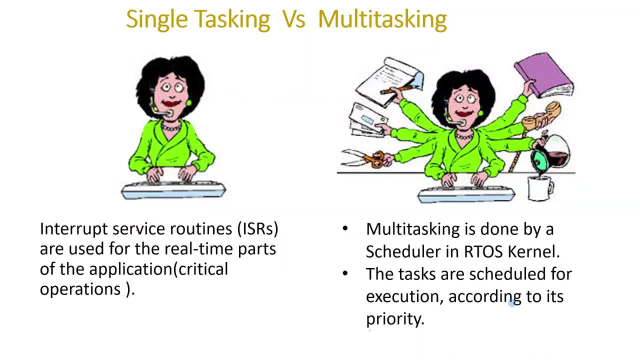 task. that is what we have been doing here with the help of interrupt service routine. with the help of interrupt service routine, we were able to do. you know, a critical section of an application may be given priority and it may be executed by skipping the main program for a small instant of time. that 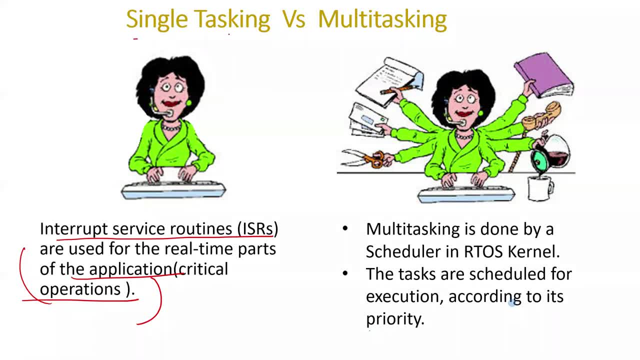 is what we have been doing so far. so, in a single tasking environment, critical sections of the core which requires immediate attention or taken care of by interrupt service routing, whereas there is a dedicated software component that is present inside an auch. does it just called as a scheduler or, alternative, is also called as kernel? 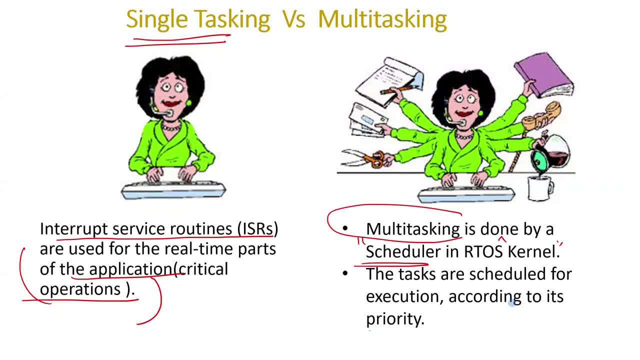 which is confirming this multitasking functionality of the artist. so which means In a single tasking environment, like we did so far, multitasking ability is very much limited, whereas in our task, multitasking is a full-fledged facility that is created by the scheduler. 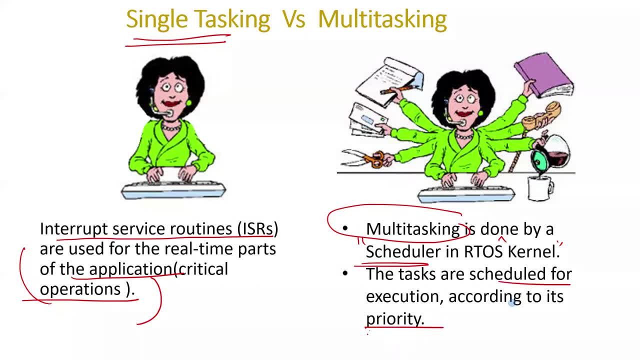 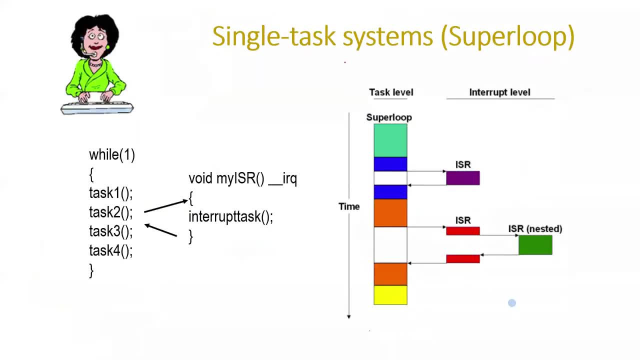 Tasks are scheduled for execution depending upon the order of their priority. That is something that you have to understand. So that is what we used in a single tasking system. In a single tasking system, we used one super loop. This is called a super loop, an infinite while loop. 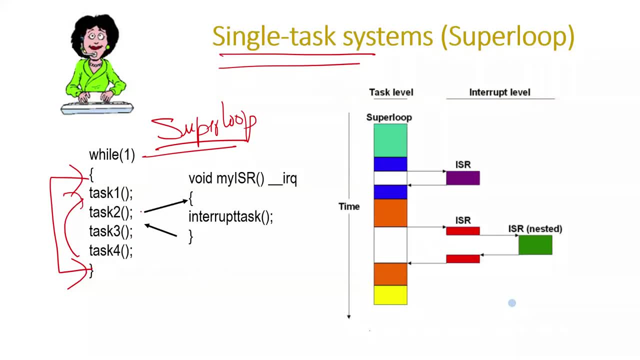 So in a super loop, the task is executed in a cyclic fashion and then, once an interrupt happens, it suddenly jumps to that interrupt service routine executes that and it comes back. So this is another timeline way of doing the same thing. The super loop is getting executed. 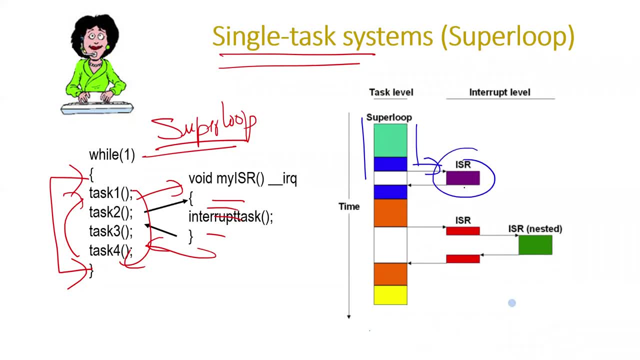 The moment an interrupt happens here, it executes the interrupt service routine and it comes back Again at some other instance. we used a super loop At some other time. when the interrupt happens and it comes back, an interrupt can again interrupt some other interrupt and it comes back. 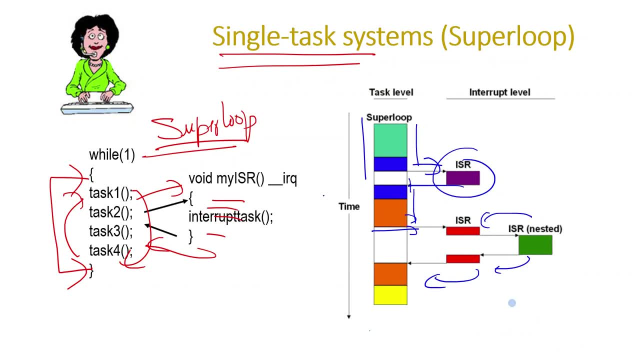 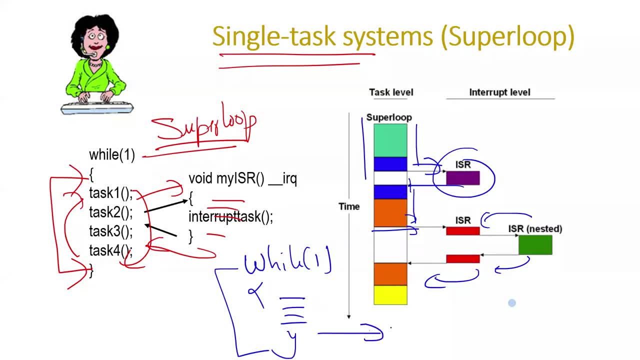 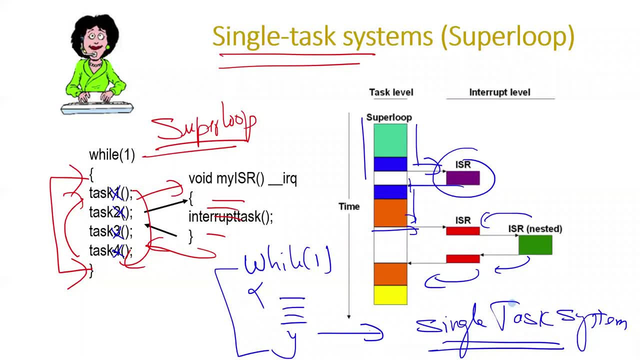 They are highly misleading. You can call them as functions. You can have n number of functions within a task. You can have n number of functions within a task. A task or a process in an application refers to an infinite while loop where multiple functions 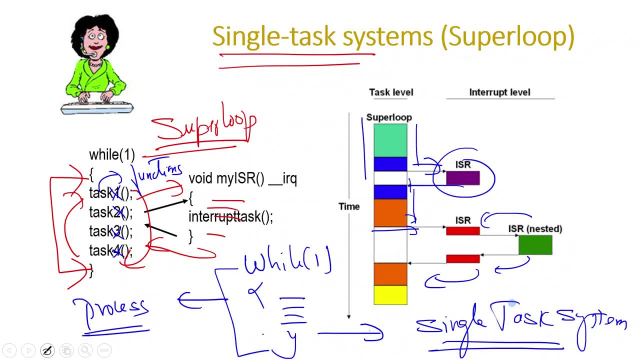 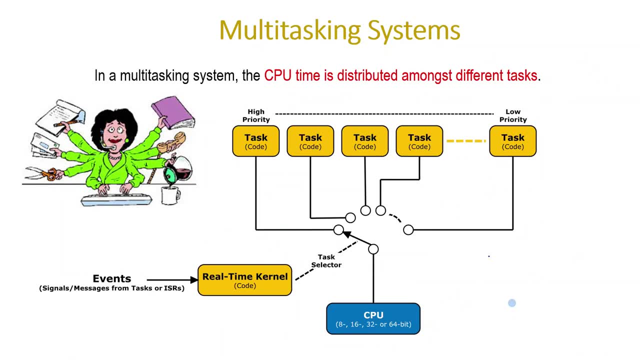 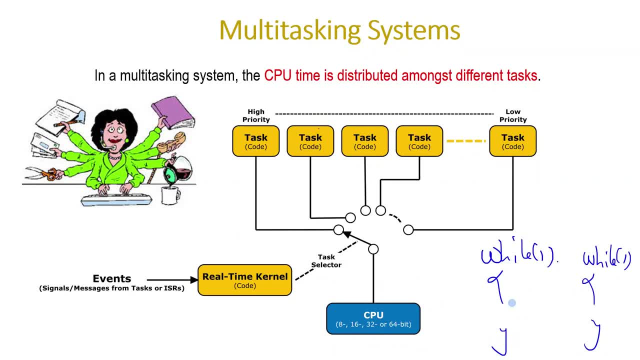 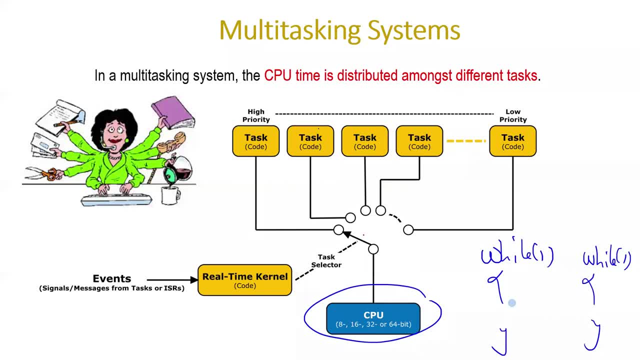 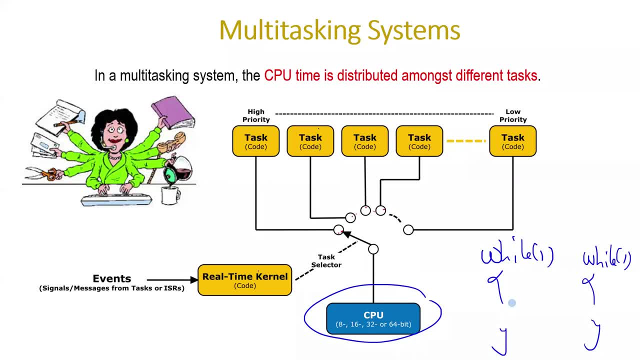 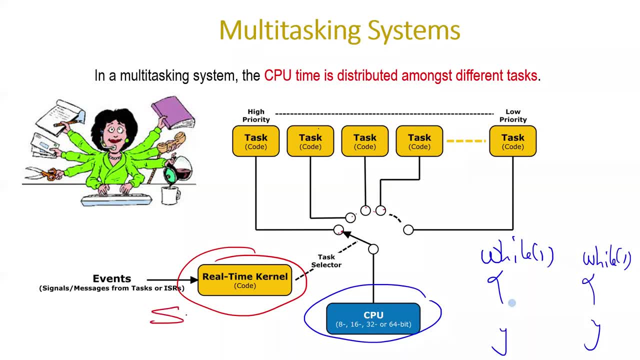 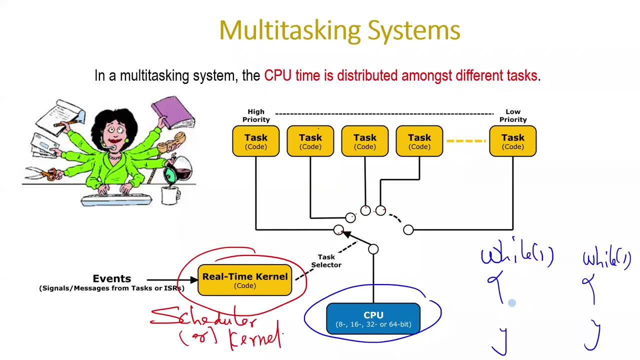 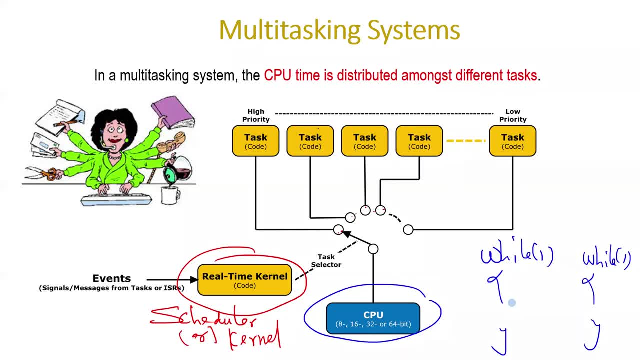 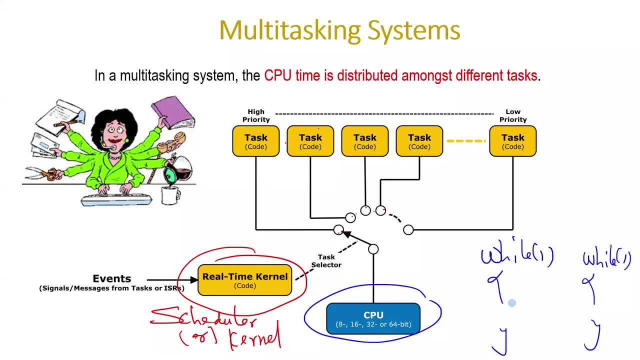 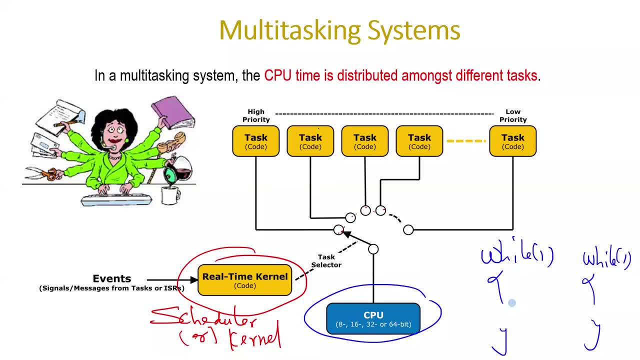 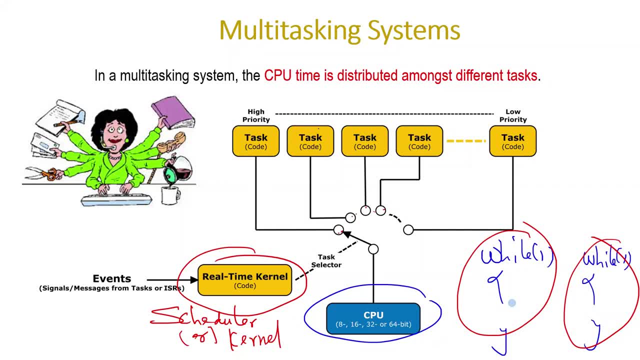 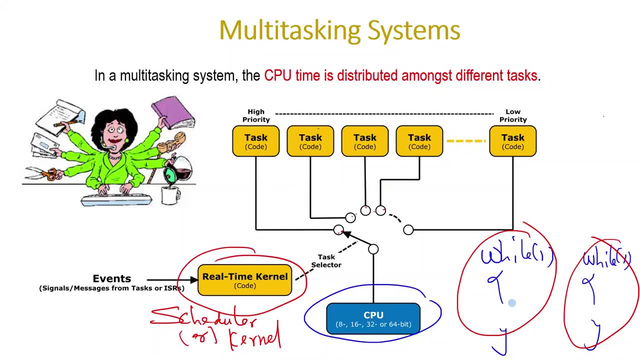 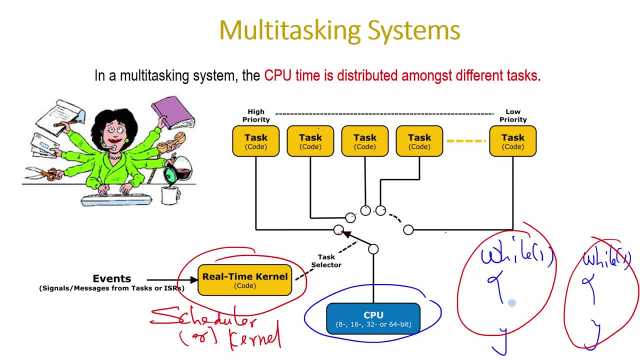 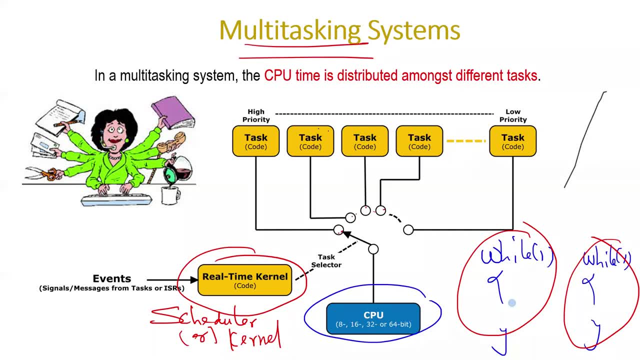 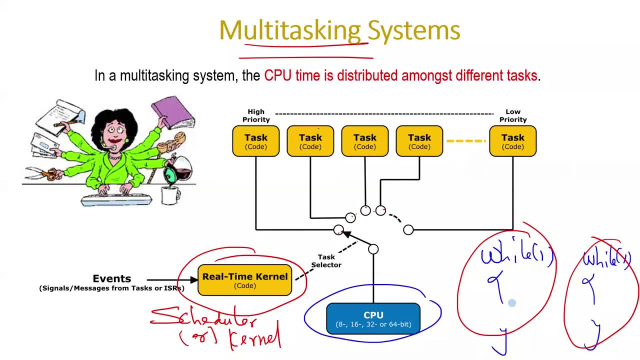 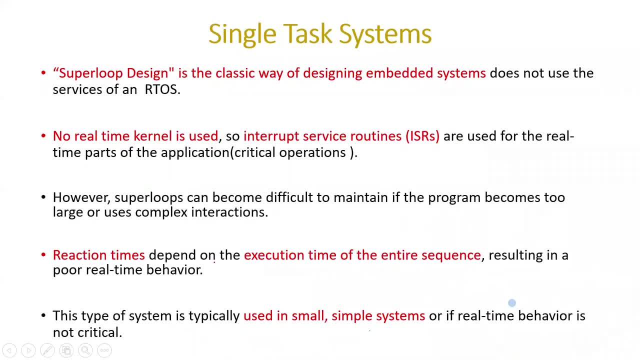 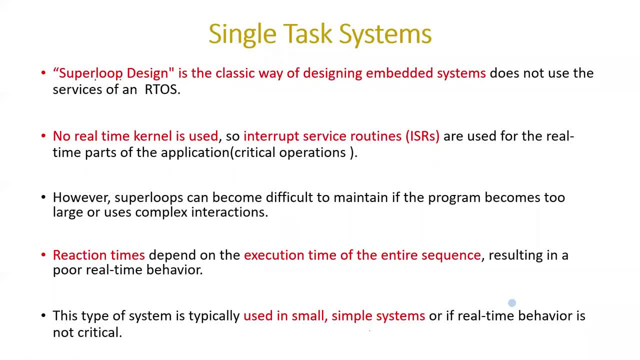 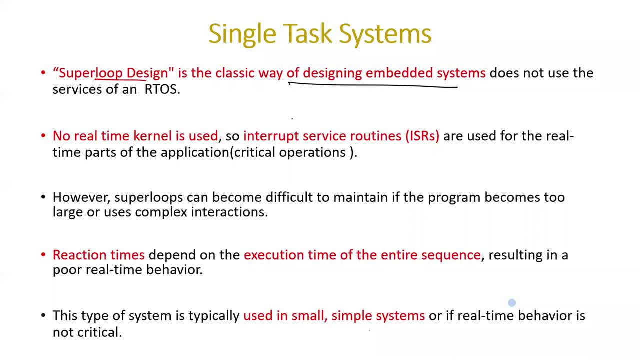 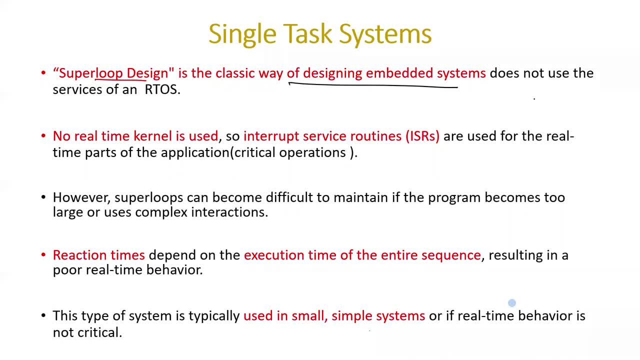 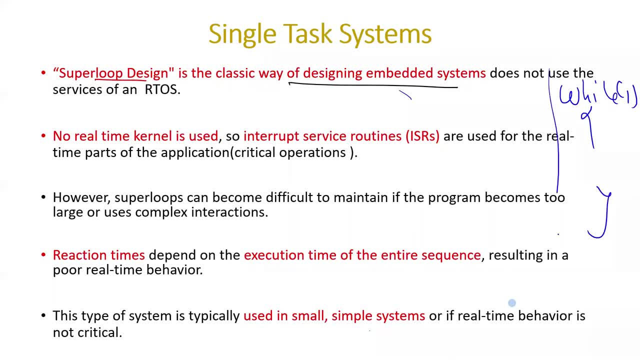 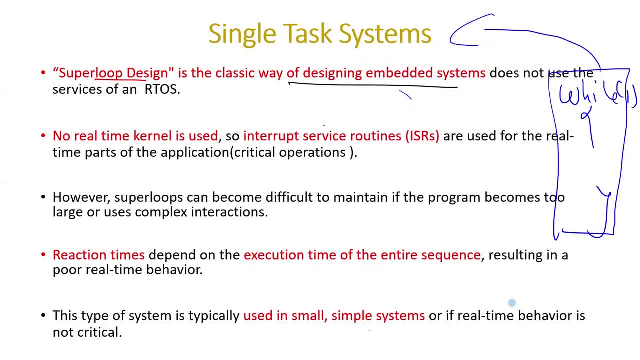 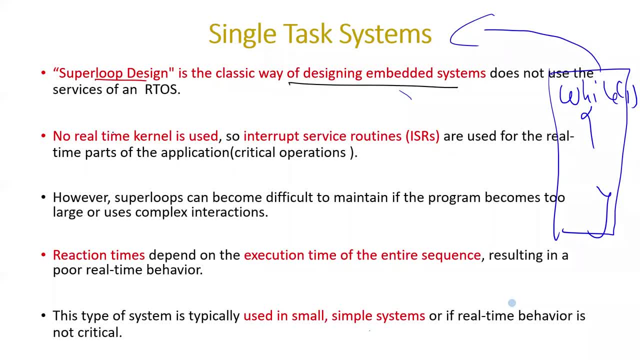 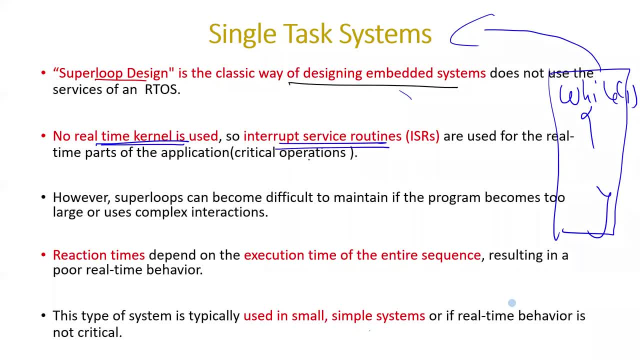 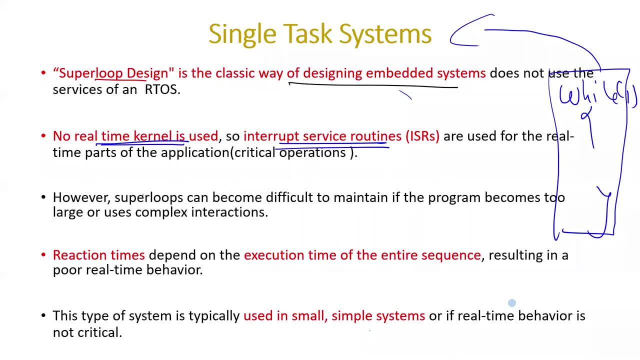 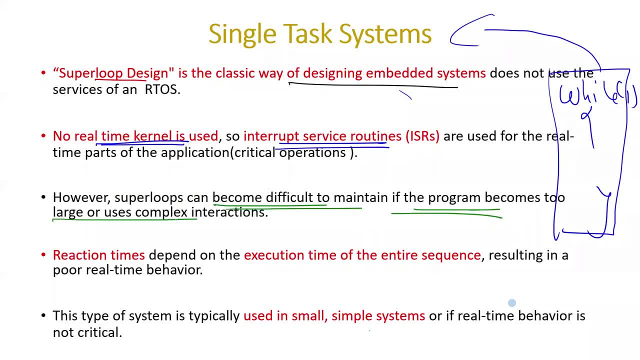 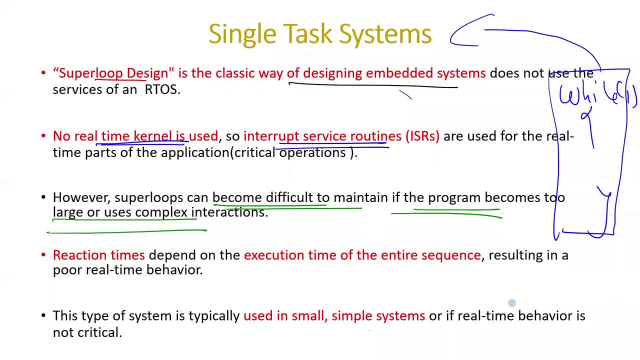 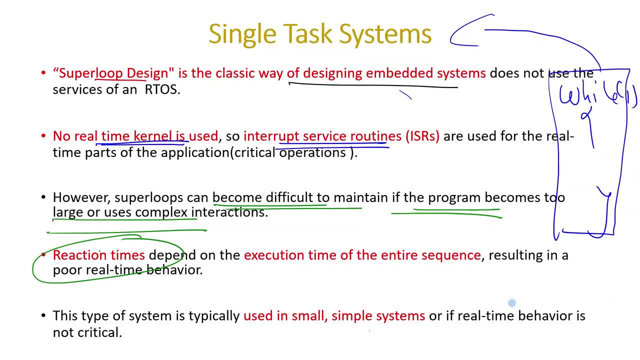 This fellow is having one while-one loop. Reaction time means what is? the ability of the system to spontaneously react to the external events is very, very minimal, which means because all the applications have to be run on a cyclic fashion, if something happens in the very first block, the reaction time or the processor attending 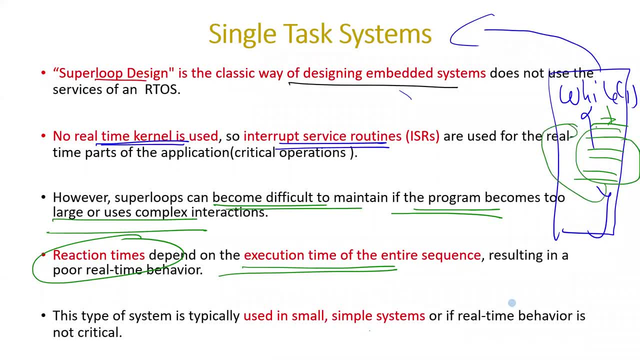 that is dependent on what is the amount of time that the rest of the functions are going to take. So the in a single task system, the system is not so reactive or it has a very poor real time behavior and, more importantly, this can be used in small and simple applications. 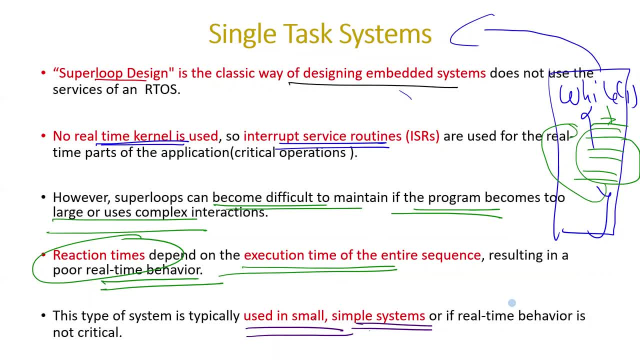 Simple IO systems- switching reading a switch and controlling a simple buzzer, performing a simple data acquisition system or doing simple applications like we did in your lab of I- can be used with single tasking systems, but when the application complexity grows, single tasking systems is of very little use for you. 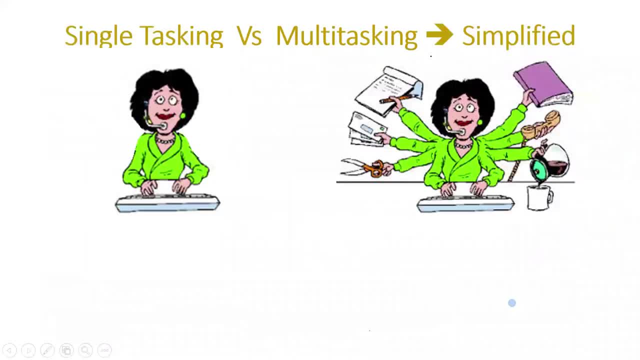 So that is something that you have to understand. So single tasking and multitasking- simplified task refers to a portion of an application. So what does it mean to be single tasking system? Single tasking means you have only one while loop. The entire application I put in a single task. that is what I mean by single tasking. 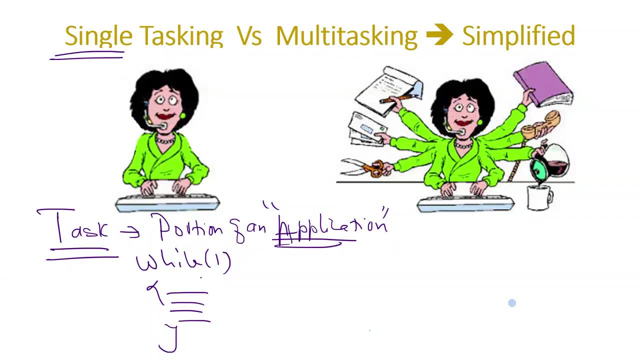 In single tasking system there is no distinction between a task and application, because the entire application I am going to put in a single task. a task here refers to one while one loop. Now, multitasking system. I am going to do a reevaluation. 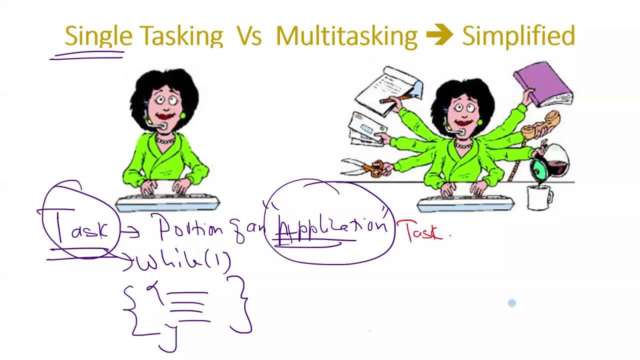 on the other hand, each task has its own, while one loop task one has its own, while one loop task two has its own, while one loop task three has its own while one loop. and there is a software component called a scheduler which executes this tasks by time, sharing the CPU's time in a 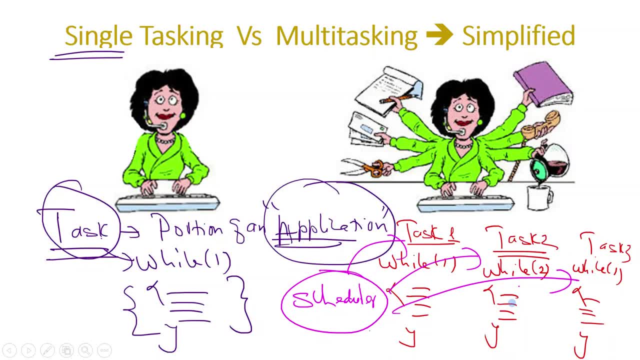 systematic manner. okay, so that is the difference between multitasking and single tasking. for a layman, single tasking means it has only one, while one loop multitasking means I divide the entire problem into multiple tasks. tasks are subsections of the application. each one I coin a name, each one I called a task, and. 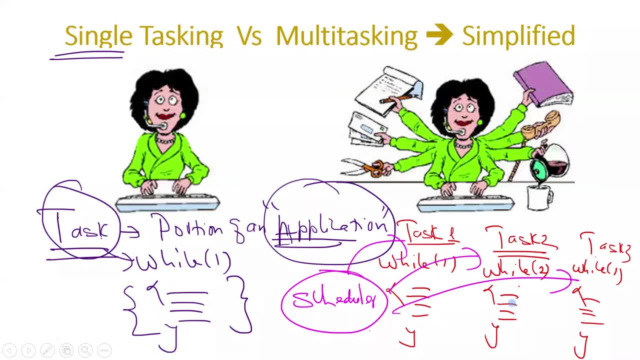 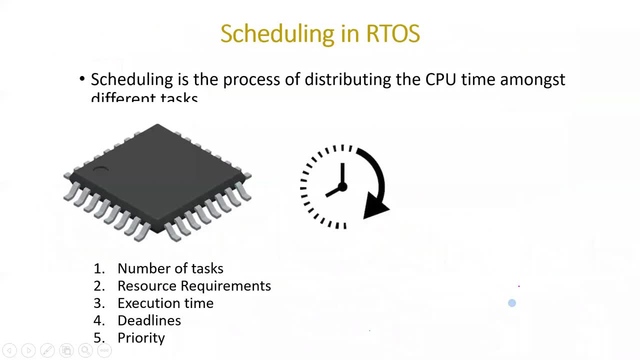 handout that asked to a scheduler to execute it in a predetermined manner. so that is the difference between the two. so what is scheduling in our tasks? scheduling in our tasks means sharing the time of the cpu versus various tasks. i have task one, i have task two. i have task three. 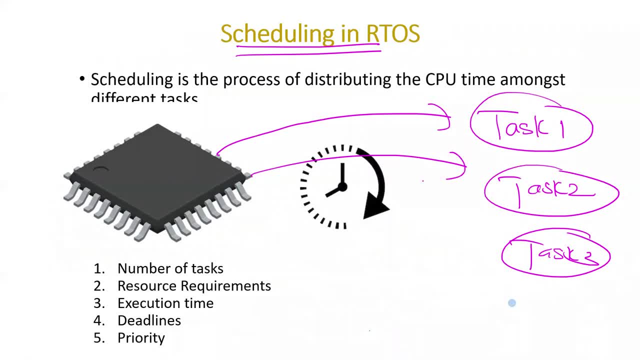 so which task should take the processor's time at any given point in time is decided by a software library or a software block called scheduler. scheduling is the process of distributing the cpus time amongst the different tasks. for some portion of the time- task one- take the ownership of the processor. this is my processor for some portion of the time. task two: 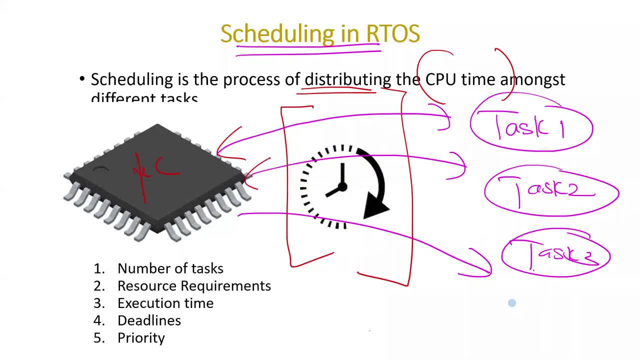 take the ownership of the processor for some other time. task three takes the ownership of the processor. so all these multiple tasks take the ownership of the processor for a specific time frame. so this process of the processor distributing the microcontroller, microcontroller or cpus time, amongst various tasks is called. 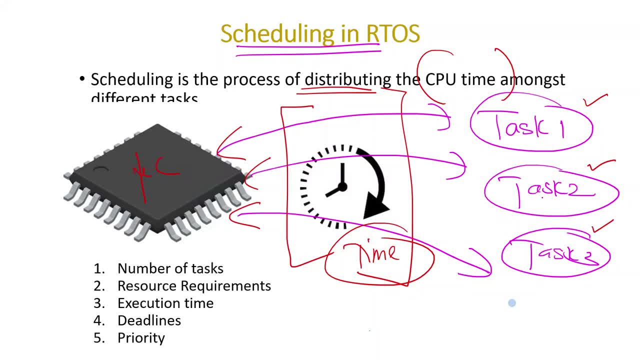 scheduling scheduler is the software which does the scheduling part. you can imagine this situation like: here is the minister, he is the pa to the minister. the job of the pa is to schedule the time of the minister for various tasks that he has to do from morning to. 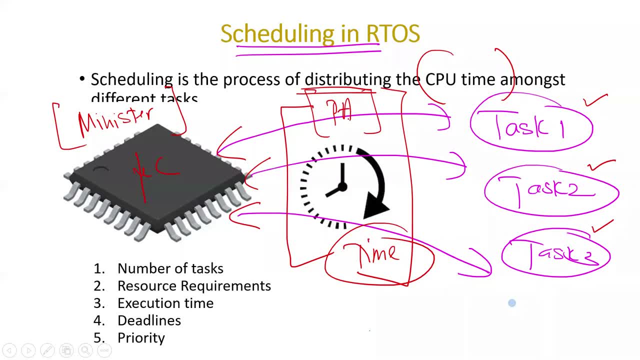 evening, from 8 o'clock to 9 o'clock. he has to do this from 9 o'clock to 10. 10 o'clock, he has to attend a meeting in the chief secretary. for 10 o'clock, 11 o'clock, he has to attend a function. 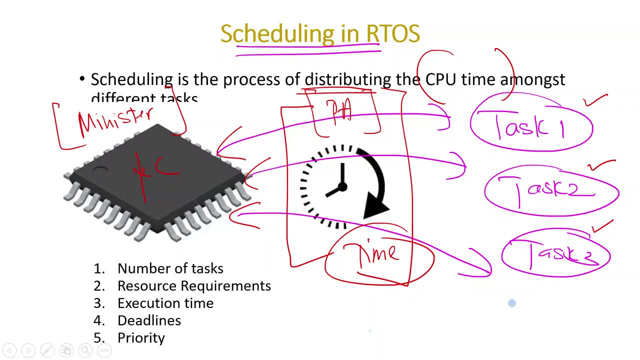 from 11 o'clock to 2 o'clock he has to do some welfare schemes. so like that he schedules all the activities of the minister at a specific priority. all the tasks are equal priority. depending upon the priority, the pa will allocate the time of the minister. 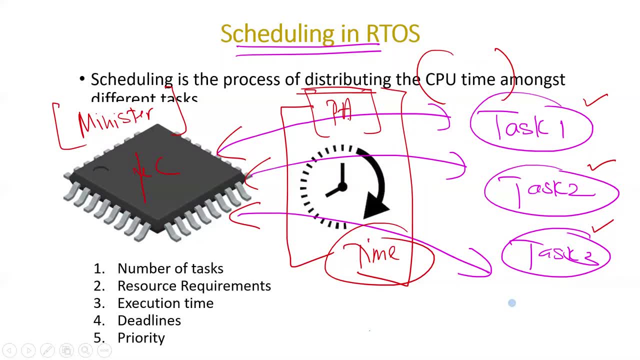 in a predetermined manner. so that is the job done by a scheduler. scheduler is something similar to the pa of a minister. minister, in this case, is the cpu. the cpu is the most precious resource. the time of the minister is very important. likewise, the time of the cpu is also very. 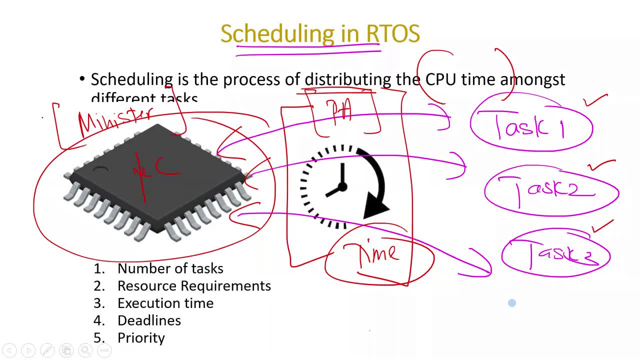 important. so the the scheduler manages the time of the cpu by allocating the time of the cpu to various tasks depending upon the priority of the task. in order to assign the time of the cpu to various tasks, the scheduler should know well in advance these five components of the task. 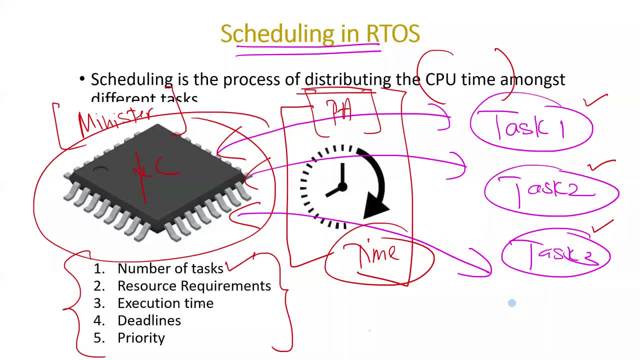 how many number of tasks that the scheduler has to execute, what is the resource requirement of each task, how much time it will take for executing one particular task, or what is execution time of it, what is the deadline needed for a task, or whether that particular task is having any time limitation or real-time constraint. 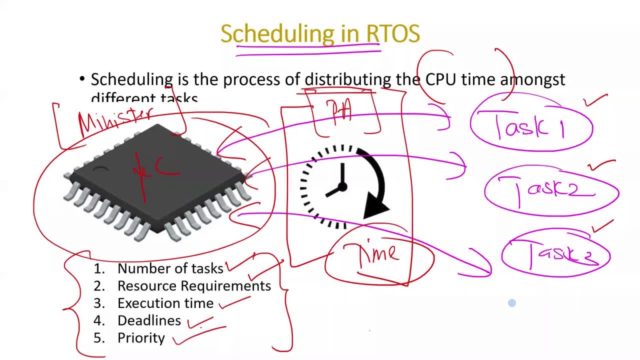 within which it has to be completed and, last but not the least, what is the priority of the task, whether it is a low priority task or a medium priority, or a high priority task. so all this information must be submitted to the scheduler well in advance. only then the scheduler can 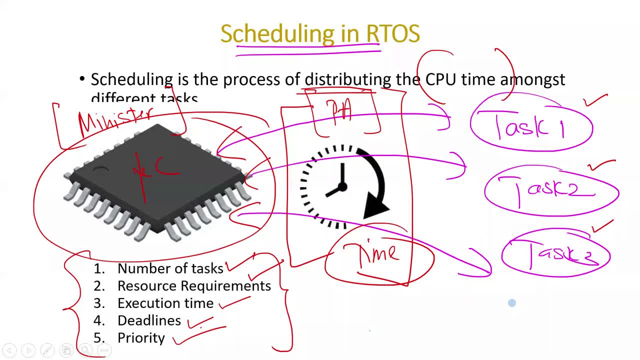 take a call accordingly and it can dispatch the task in a given preference in the order of their priority. otherwise it will be a total miss. say, for example, the task one can be a chief mistress meeting and the task three can be a simple wedding ceremony that he has to attempt. so if the, if the pa doesn't know how to prioritize between these two, 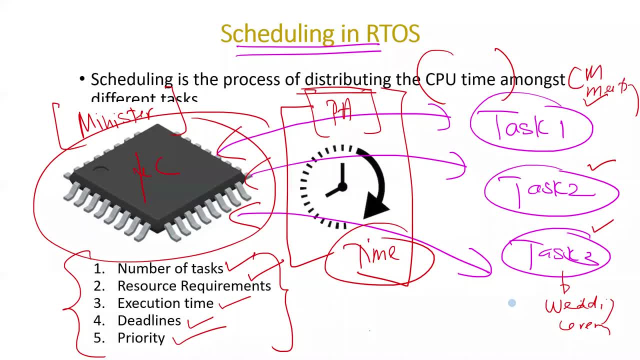 and he assumes that all the tasks are having equal priority. and if he is scheduling the minister's time for a wedding ceremony instead of attending the meeting with CM, probably it will result in a bad consequence. So that is how it is. So in a real time system. 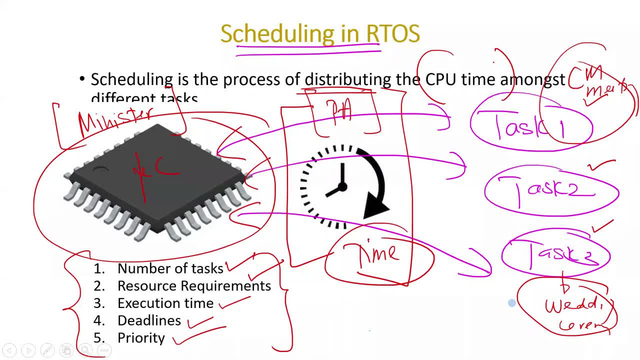 we cannot give equal priority to all the tasks. For example, in a car example, the airbag always takes high priority over rest of the tasks. When some accident happens, the microcontroller should address to that immediately, no matter what happens, Otherwise the driver is gone. So 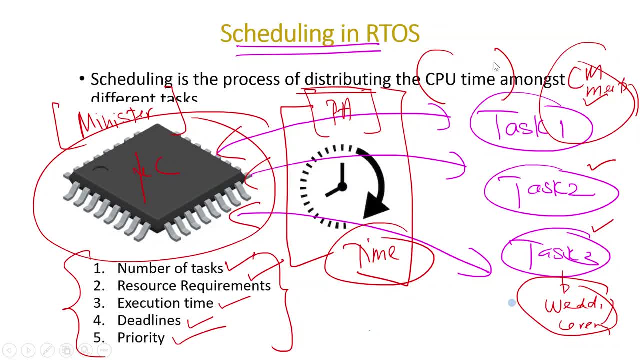 the scheduler inside the real time operating system of the car will always give high priority to airbag system. So when a signal comes from the airbag system, it will suspend all the other activities and spontaneously go and react to it. So that is what we mean by prioritizing. 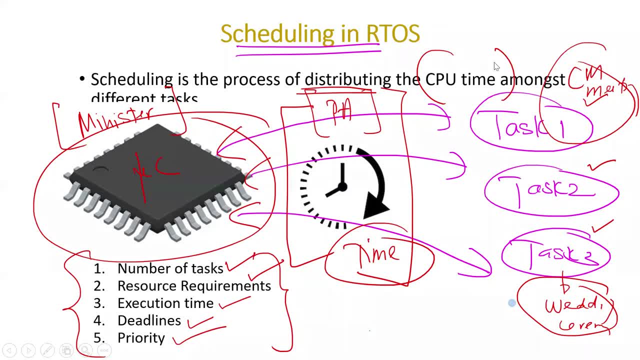 a task, Though it is possible to handle this with interrupts in a traditional embedded system, which we have been doing so far, they are not reliable. They are not reliable means there is no guarantee that it will go and execute in a given timeframe. So 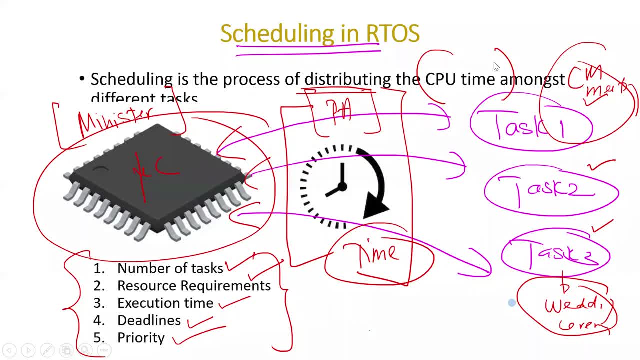 interrupts are unreliable. There is no guarantee that they will execute And, moreover, if you have a complex system which involves a lot of such high priority tasks to be executed, interrupts are not a reliable way of doing it, So using a real time operating system becomes mandatory in such a case. 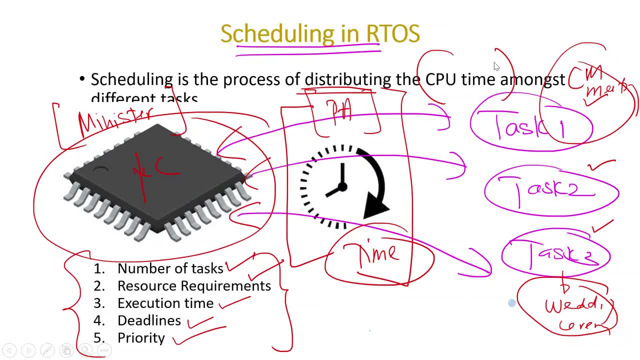 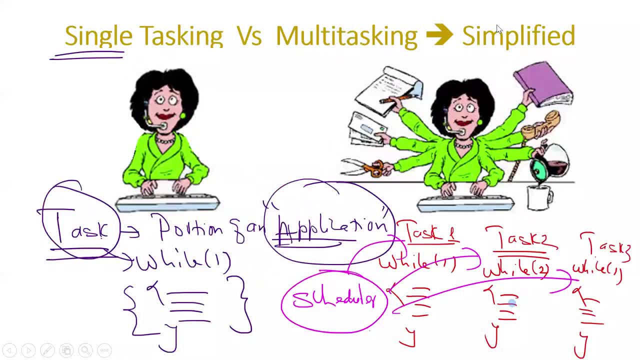 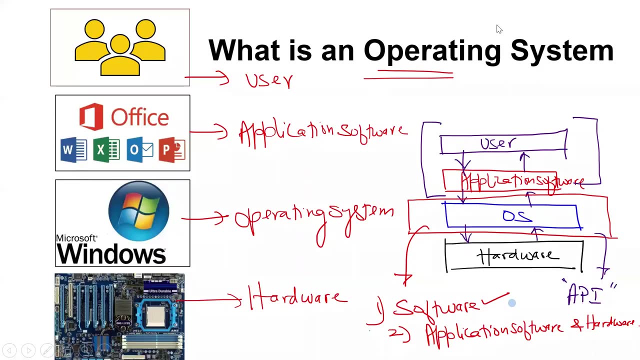 So I stop here, Though I have a lot of concepts to discuss, today being an introductory session, I stop here, So I will quickly revise what we discussed today before we move further. So we saw what is an operating system. An operating system essentially consists of a software block. 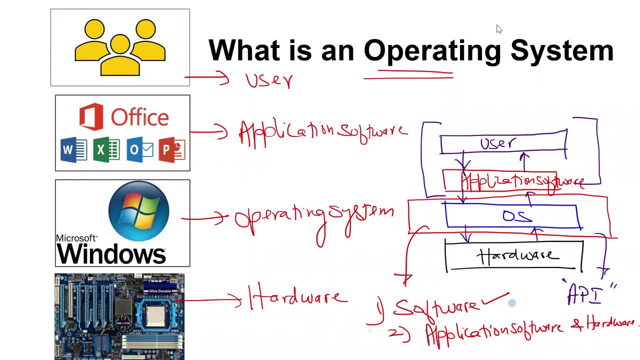 which is acting as an intermediate layer between the application software and the hardware. So it is always possible to control the hardware directly by using an application software. But it will make the life of an application software developer miserable because he has to manage all the underlying hardware complexities on his own. So a software 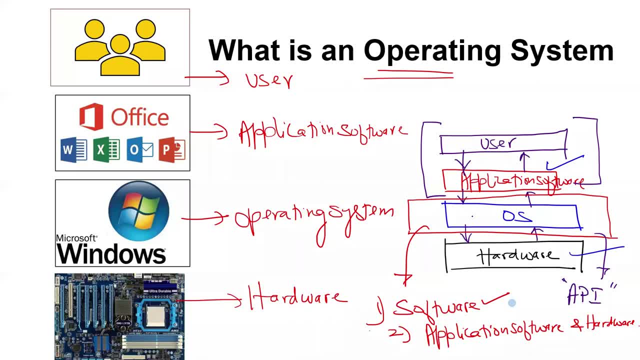 an intermediary software in the form of an operating system does the job of providing set of APIs for the application developer so that he makes the application development with much ease, because all the hardware complexities are taken care of by the operating system. So in the entire chain. 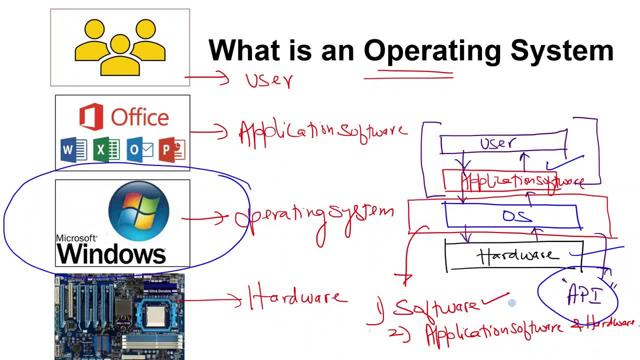 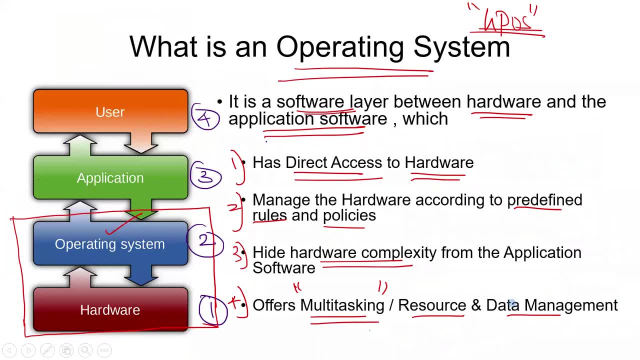 the operating system fits somewhere in between the application software and the hardware, So it is essentially a software that you have to understand. This software architecture of an operating system does the following things: It has direct access to hardware. It manages the hardware at a. 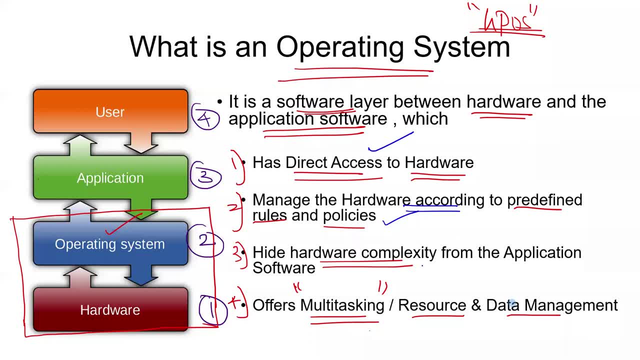 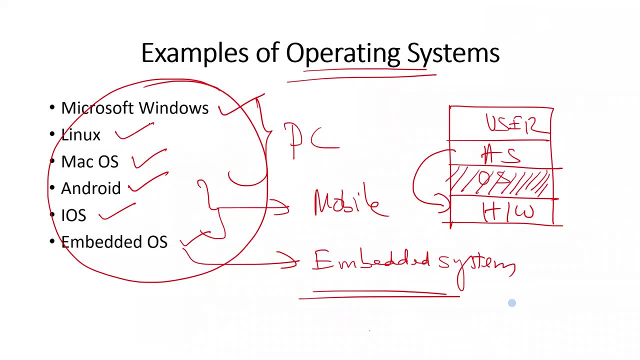 predetermined rules and policies. It manages or hides the hardware complexity from the application software. Last but not the least, it offers multitasking capability. So examples of operating systems are: for PC, it is Windows and Linux. For mobile devices, it is Android and iOS. For embedded systems, it is embedded OS. 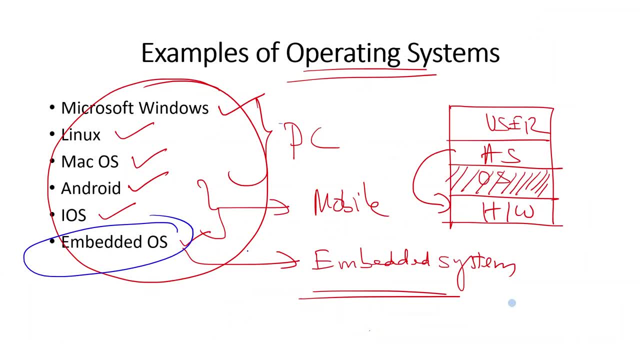 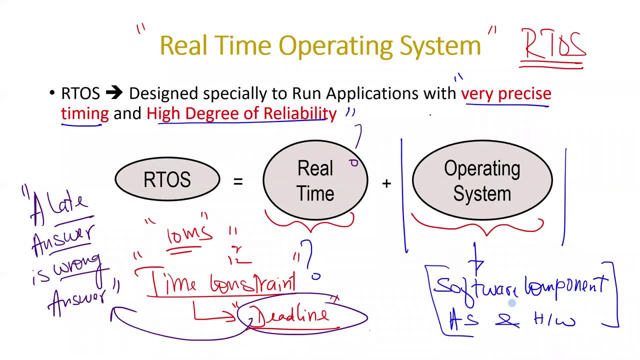 Lot of embedded operating systems are there. We will see them in later classes. This is the definition of a general operating system For real time operating system. it is an operating system with some special characters. What is that character? That character is a real time character. Real time character means what? 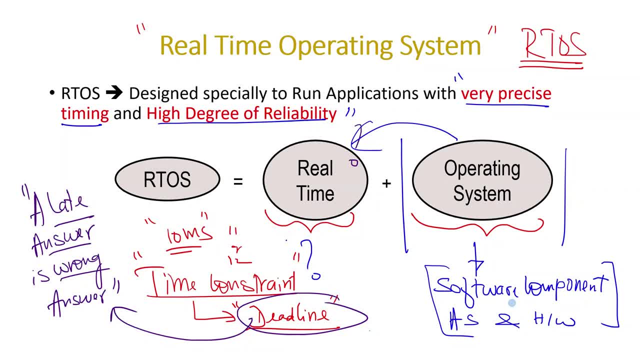 It is the ability of an operating system to perform an application with a time constraint. Time constraint means what? If it is supposed to perform something at a predetermined deadline, it is supposed to do it within the deadline. That is what we mean by real time capability. Real time capability. 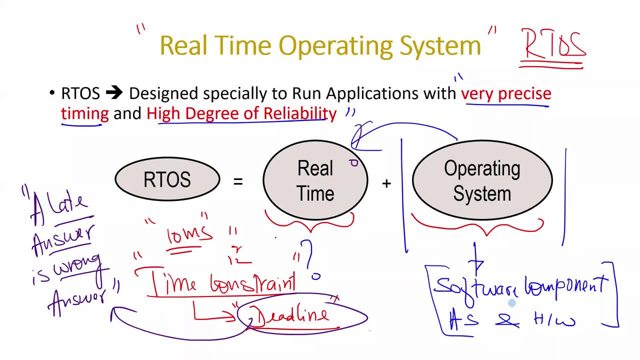 means the ability of an operating system to perform an application at a predetermined time constraint. That is what I said. A late answer is a wrong answer. in real time scenario, If the system is able to deliver proper results but not at a specific time interval means it is considered as a wrong answer. 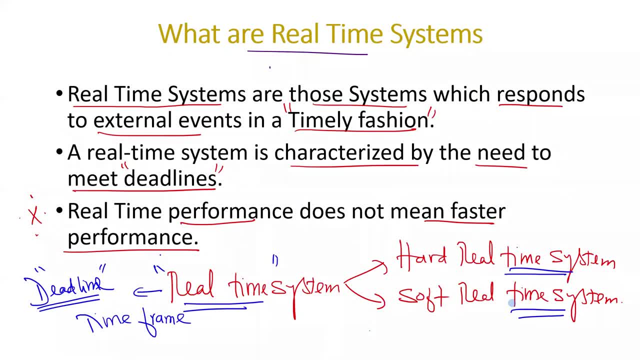 So what are the real time systems feature In a real time system? systems are expected to deliver results in a timely fashion. It is expected to meet deadlines. A real time system doesn't mean that it offers faster performance. Say, for example, I have two systems: System 1: 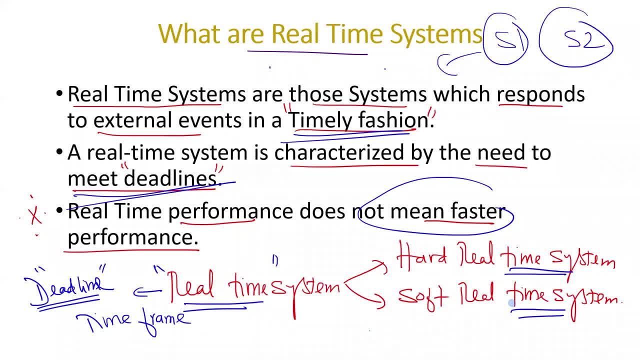 System 2.. System 1 is operating at 1 kHz. System 2 is operating at 10 MHz. Just because a system is operating at higher speed, it doesn't mean that this is a real time system and it is not a real time system. So the operating. 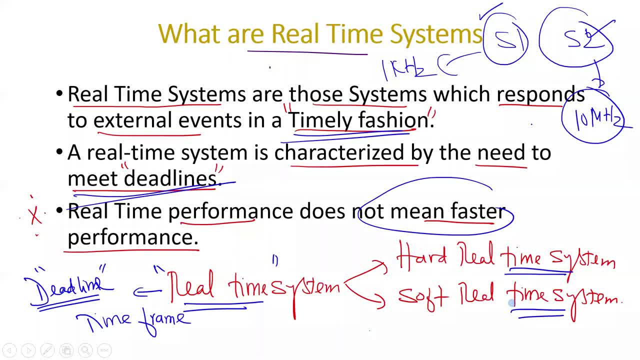 frequency or the rate at which the system is operating is not the criteria for real time system. The criteria that decides whether system 1 and system 2 are real time system is whether they are able to meet the output, Whether they are able to deliver the output. 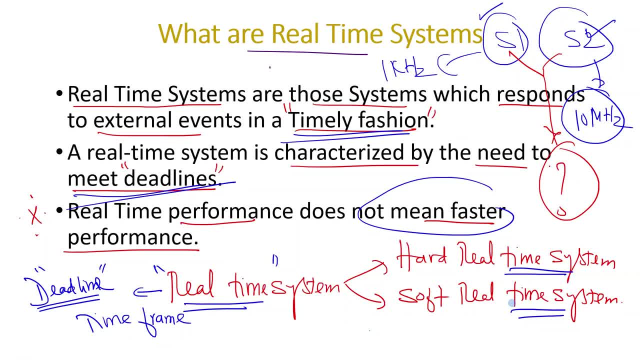 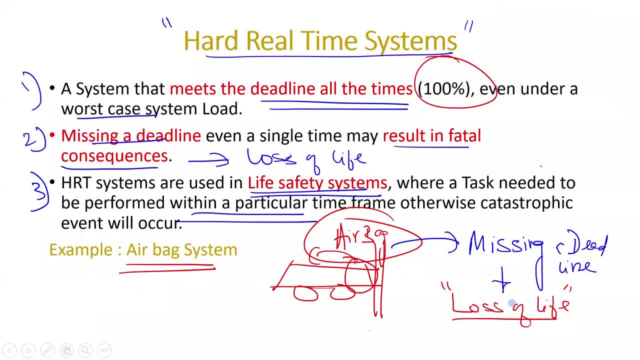 well within the deadline or not. Deadline depends upon the type of the application. Not necessarily it has to be fast all the times, That clear understanding you have to have. So we classified real time into two. One is hard real time system and the 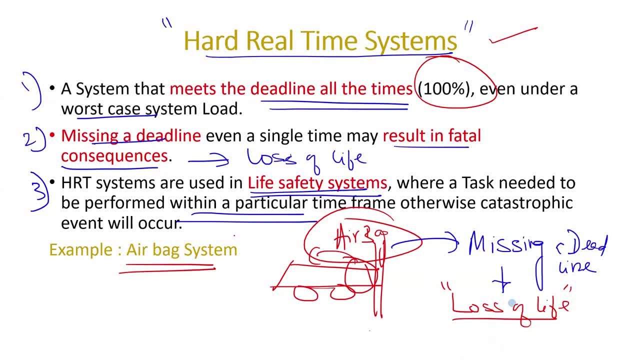 soft real time system. Hard real time system: the best example is the RBAG system. In hard real time system, in 100% of the cases, the system has to meet the deadline all the time. Missing a deadline means it results in a catastrophic outcome: Loss of life. 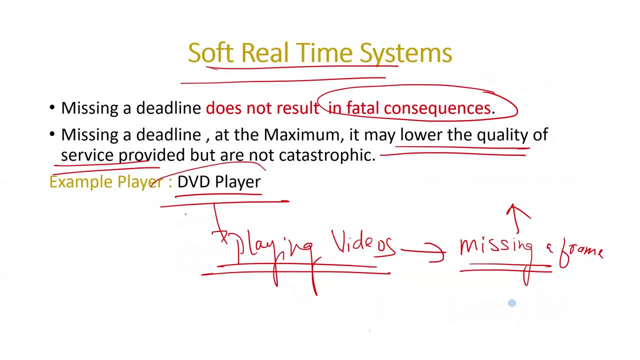 In soft real time system you can always imagine a DVD player. missing a deadline may give you unpleasant outcome, Lowering the quality of the service provided by the system, but it is not going to give you fatal consequence. It is not going to give you loss of life So hard versus. 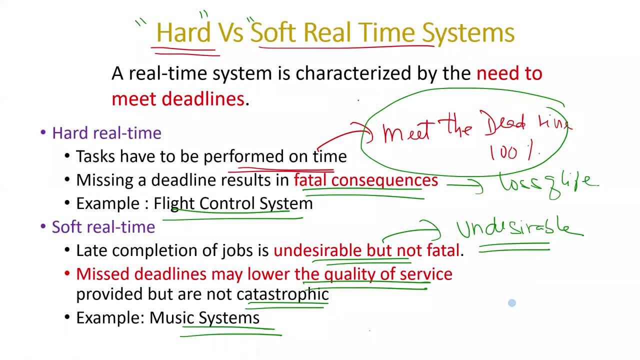 soft. here is the difference. One must meet the deadline in 100% of the cases, Otherwise it results in loss of life. In other case it will give you undesirable outcome. It will lead to deterioration of quality of the service, But it is not catastrophic or it doesn't lead to loss of life. 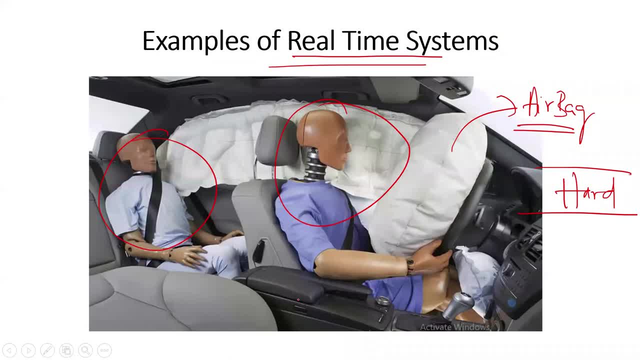 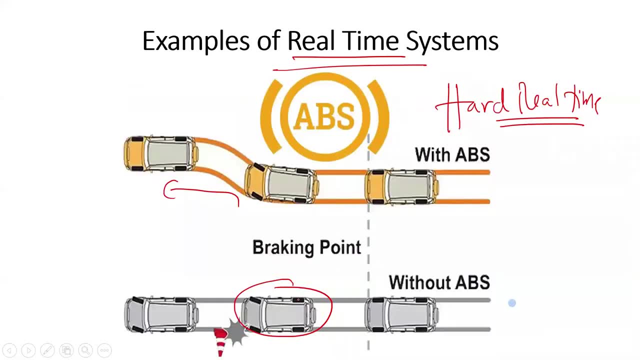 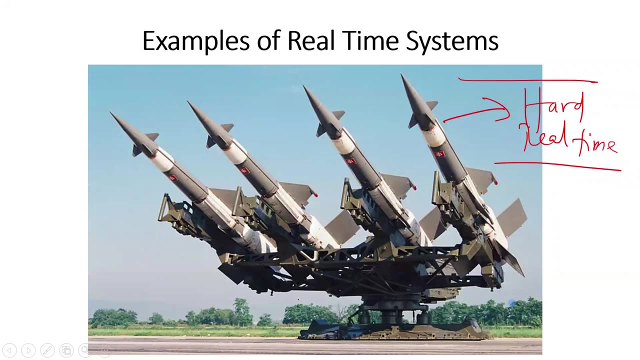 We saw some examples of hard real time systems. Number one is the RBAG system of the car Pacemaker. another hard real time system: Anti-lock braking systems or ABS systems. another hard real time system: Missile tracking and control systems. Hard core real time. 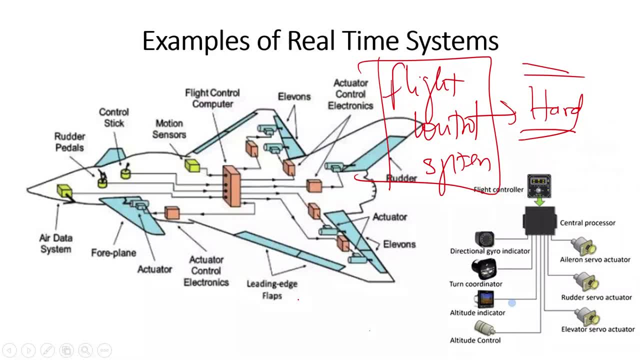 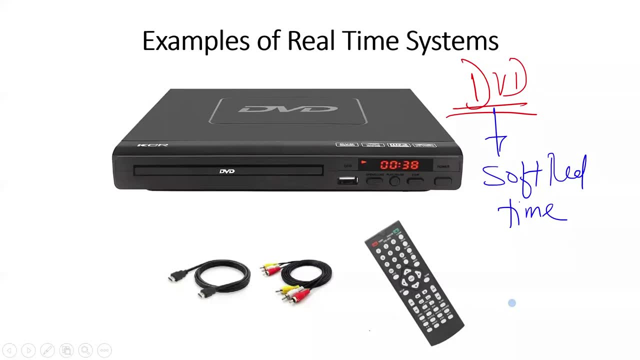 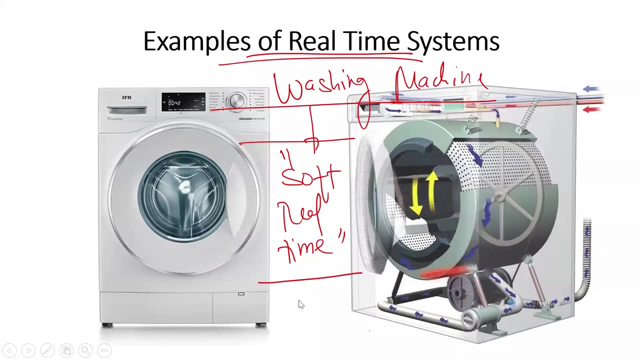 embedded systems, Flight control systems, Another hard real time system. These are all examples of soft real time systems. DVD players, Musical systems, Digital cameras, Gaming consoles, All multimedia devices will come under that category. The washing machine- again a soft real time. 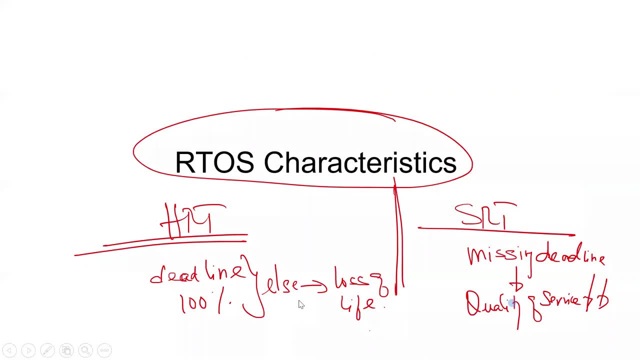 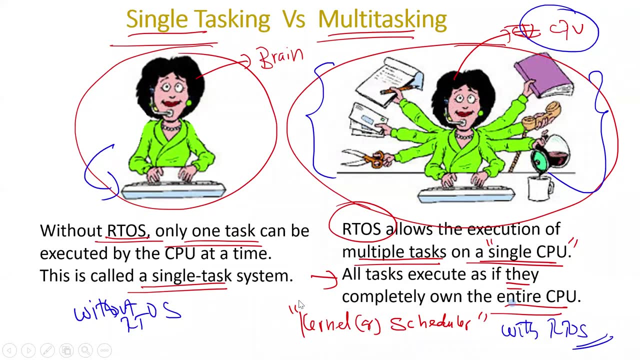 system. We saw the characteristic features of real time embedded system. We saw what is single tasking and what is multi tasking. Single tasking means the entire application is done as a single task. Multi tasking means the entire application is divided into smaller. 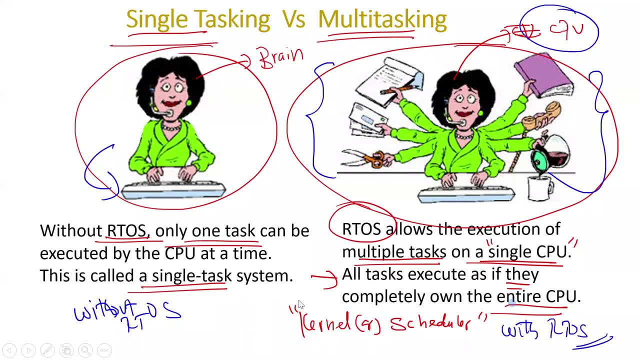 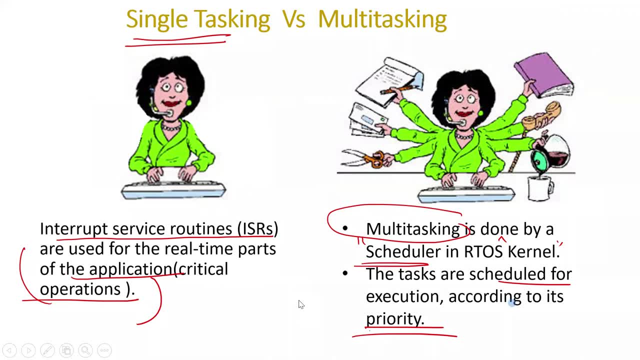 sections called tasks, and they are executed and scheduled by a software block called a scheduler. It is possible to do multi tasking in a single tasking environment by using interrupt service routine, but that is not reliable. That is the reason why 70% of the real time applications are designed by using 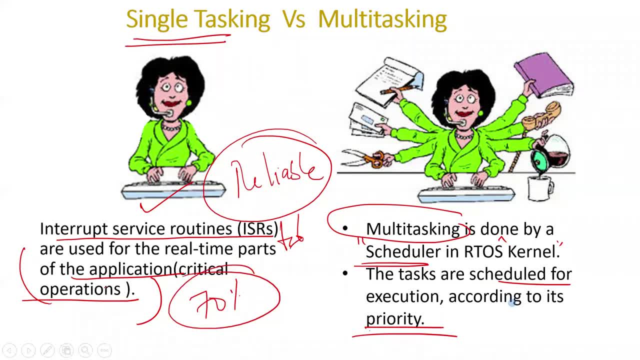 RTOS. All real world applications uses RTOS and people doesn't use interrupts for that. Multi tasking is achieved by the help of scheduler in a real time operating system which executes the task in the order of their priority. Priority means what is the importance of that? 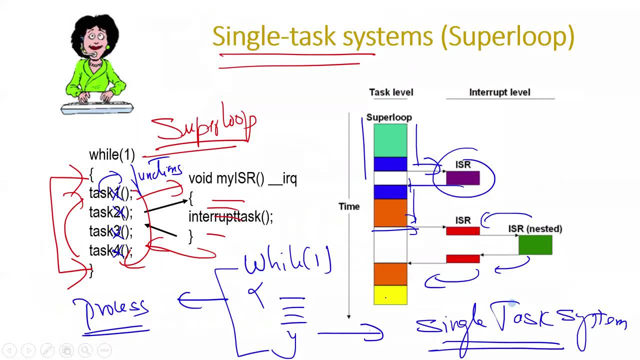 particular task. So this is how we saw. in a single tasking system, the entire application goes in a single while one loop. So this is my application. In a single tasking system, my application and task has the same meaning, Whatever goes inside one while one loop. 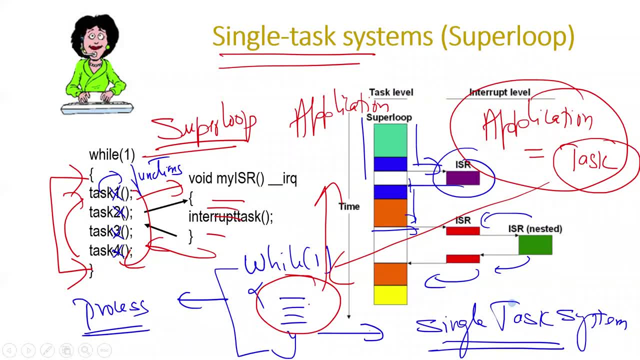 we call as a task, Since the entire application goes inside in a single, while one loop. in a single tasking system, the entire application is referred as one task. That is why we call as a single tasking system In a single tasking system. 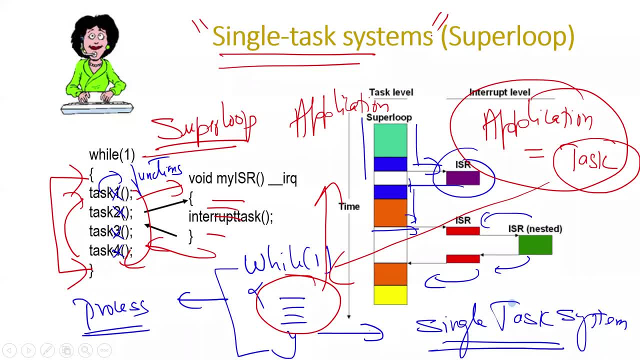 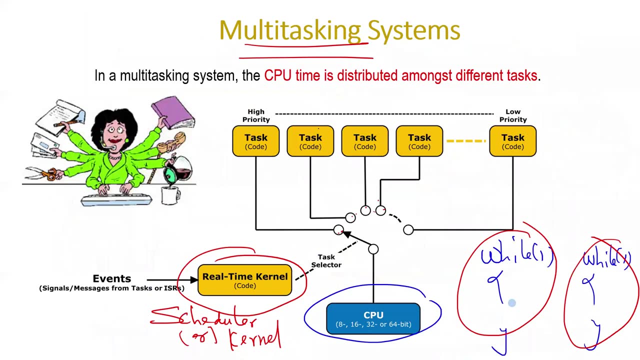 safety critical applications or time critical applications are always dealt by using interrupt service routines, but they are not that helpful when the complexity of the system is higher. In a multiple tasking system or multi tasking system, the entire application is divided into multiple tasks: Task one, task two, task three. 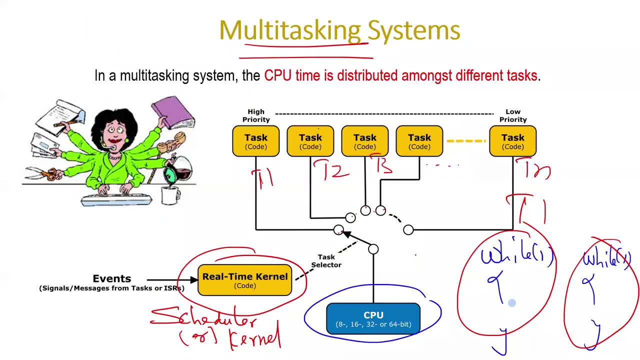 etc. up to task n. Each task maintain their own while one loop. That is the difference. You can say: how can a microcontroller can have multiple while one loops? The moment it gets into a while one loop, it is going to get struck indefinitely. 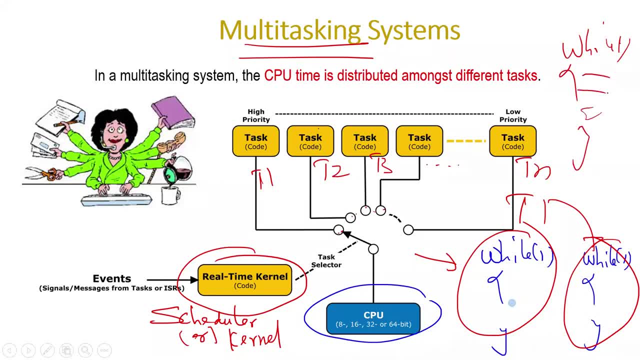 inside. How come a microcontroller can go to another while one loop, you may ask, But that is the job of a real time kernel or a scheduler, So you don't have to worry about it. Make sure that the microcontroller comes out of that particular while one loop and 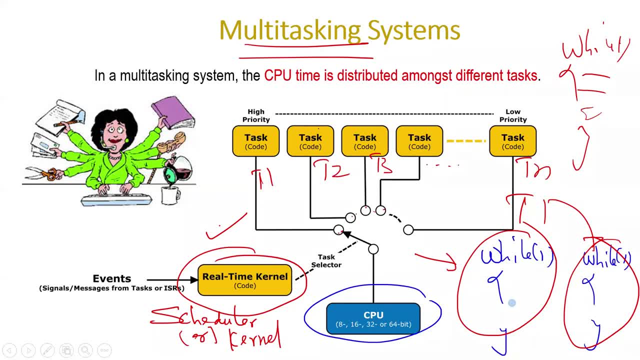 gets into another, while one loop and it executes another task till a particular time frame, depending upon the priority that you set. So that is why we take the help of our task. Otherwise we don't take the help of it. So a scheduler or a 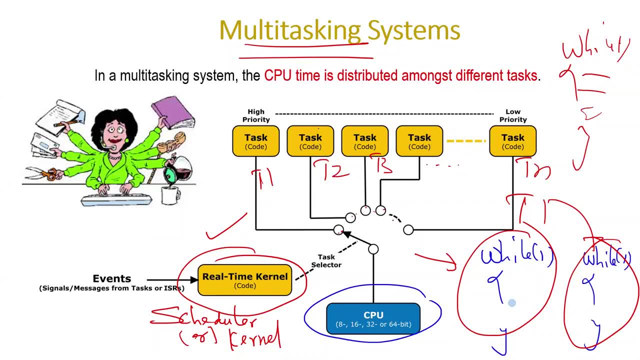 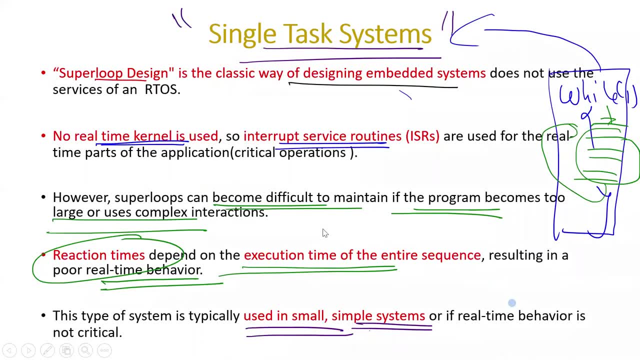 real time kernel does the job of time sharing the processor to various tasks depending upon the priority. Single tasking system always uses super loops. Super loop means one while one loop. It never uses real time kernel. It uses interrupt service routine to do some kind of a multitasking. 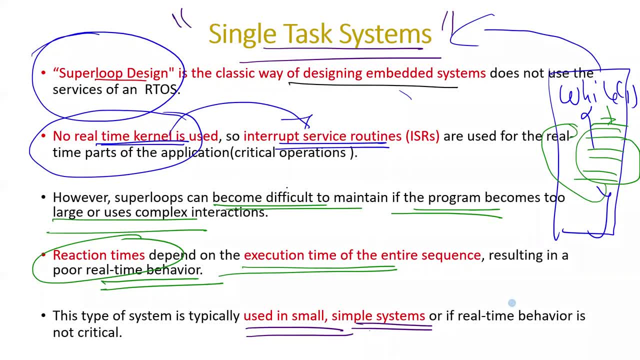 but that is not reliable. Super loops are always difficult when the program size become larger or for larger systems. The most important difficulty or disadvantage in super loop or single tasking system is the reaction time. Reaction time is how fast the system is able to react for 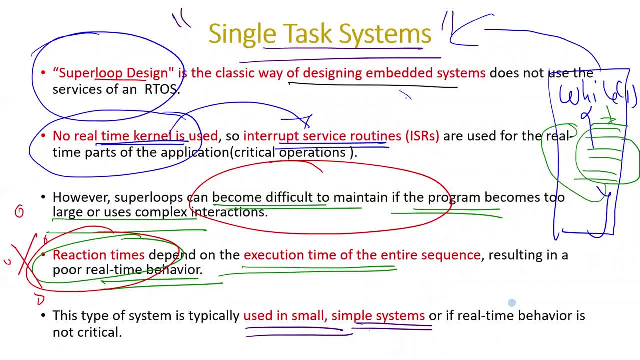 the external event. Since the application is built around a single while one loop, any event happening in the top section of the while one loop can be executed only when the bottom section is complete, Which means it has a very poor real time behavior or a reaction time. And, last but, 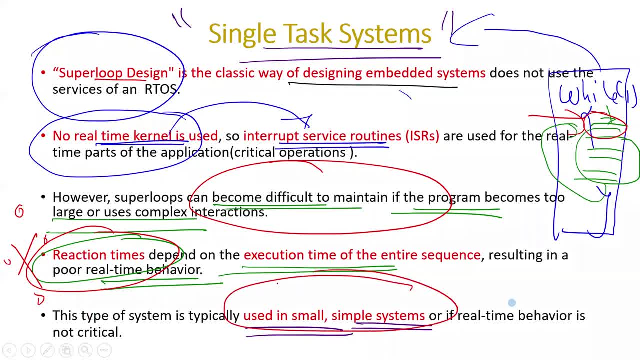 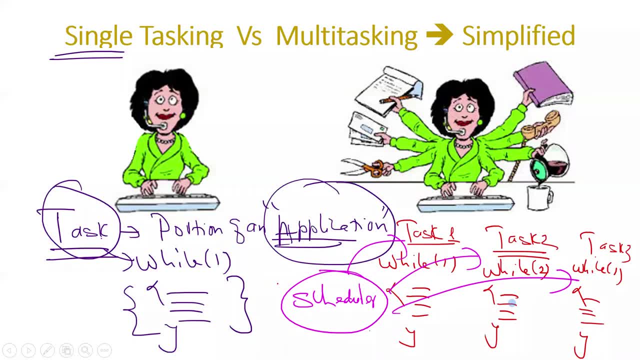 not the least, it can be used in very simple systems: Single tasking and multitasking in a simplified format for a layman. In a single tasking system, the entire application is put inside only within a single, while one loop. In a multitasking system, each task. 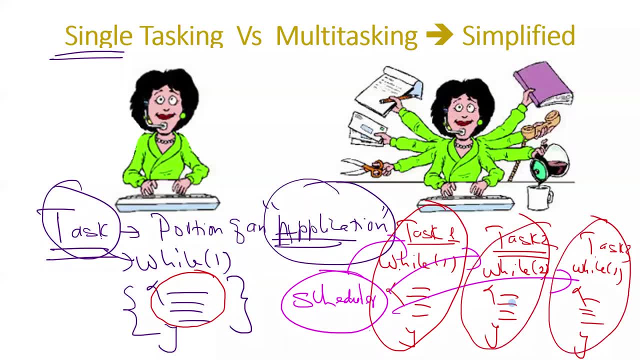 is allocated a separate while one loop And there is a block called a scheduler which makes the processor to execute this task depending upon the order of the priority. It is called single tasking because the entire application goes in a single while, one loop. So that is a simplified format. 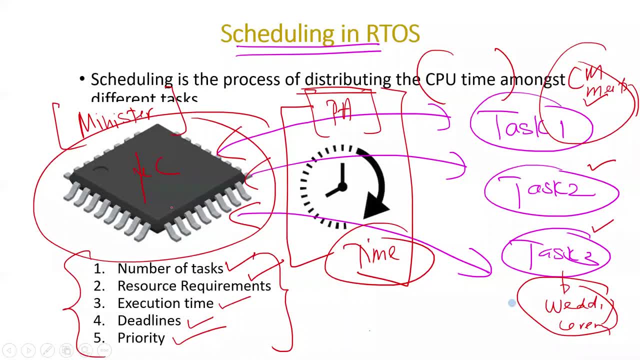 of single tasking and multitasking. Scheduling means it is a process of distributing the processor's time to various tasks. The process of scheduling is done by a software called scheduler. Scheduler and scheduling are two different things. Scheduler performs scheduling. Scheduling is an act of distributing the 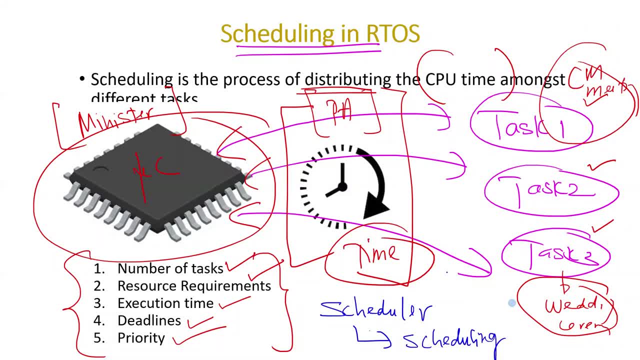 processor's time to various tasks. It is a methodology or a process. Scheduler is the person who does that, Who does scheduling? It is the scheduler. Scheduling is the process. That is why I gave the example of a minister and the PA. 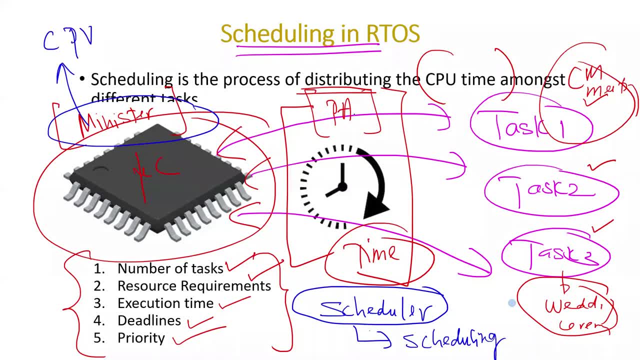 Minister is my CPU Scheduler in this case is the PA. PA performs scheduling for the CPU, So he manages the time of the minister for various tasks. In order to perform scheduling, the scheduler should know upfront all these five basic behaviors of the task.